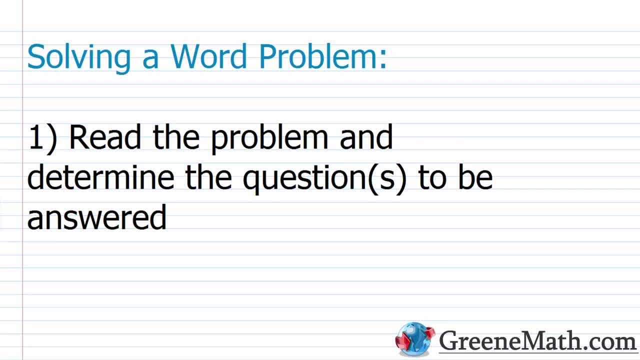 six step procedure that we used in our section on applications of linear equations. So again for solving a word problem, the first thing we want to do is read the problem and determine the question or questions to be answered. Then the next thing we want to do is assign a variable. 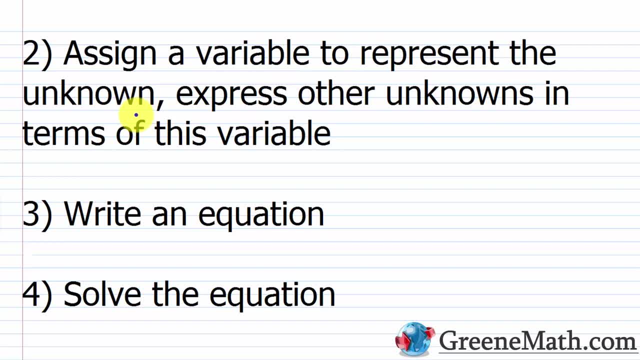 to represent the unknown and for the scenarios we're going to have today, we can express other unknowns in terms of this variable. Then the next thing we want to do is write an equation, and this is based on the scenario we're given. Then we want to solve the equation, Then we want to write: 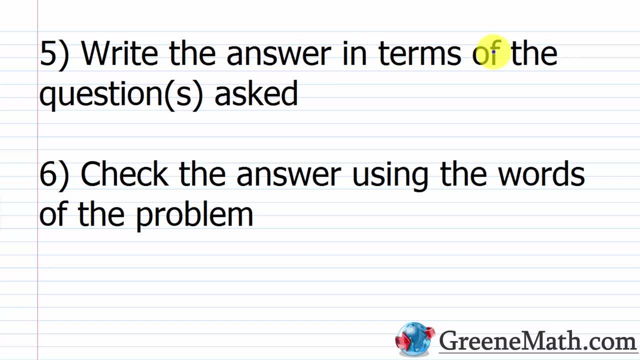 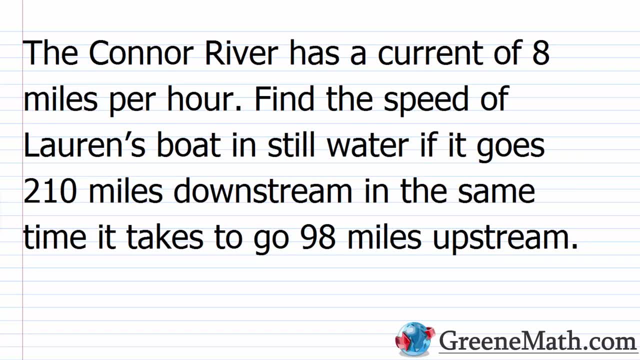 the answer in terms of the question or again questions asked. Then, lastly, we want to check the answer using the words of the problem. Just make sure that things are reasonable. So if you're in the section on applications of rational expressions, the most common problems- 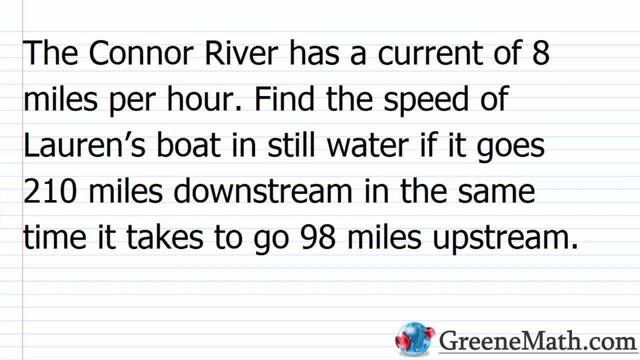 you're going to see are going to be work rate problems, or some people call them rate of work problems, or you're going to see motion work problems. right, These involve again the distance formula. distance equals rate of speed, times time travel. Okay, So we talked about this. 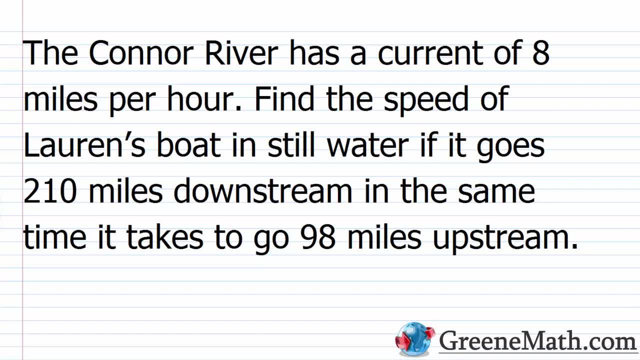 formula when we looked at applications of linear equations. So we see it again. Okay, And we'll see this throughout our course many times. So again, if you don't know, the formula d for distance is equal to r for rate times, t for time. So if I'm going 40 miles per hour and I do this for three, 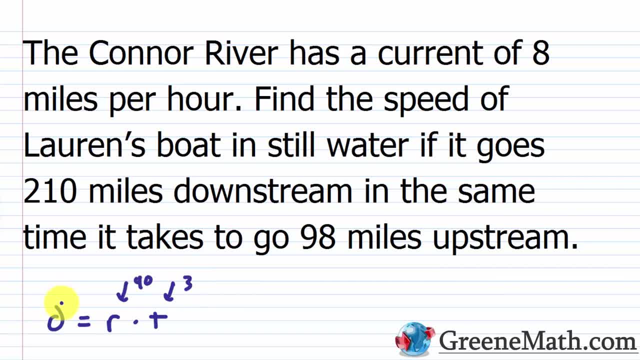 hours. I multiply 40 times three, that gives me my distance of 120 miles. Okay, so this would be 120 in that case. So pretty easy formula to understand, Very, very intuitive, And we're just going to use it to kind of solve this first problem. 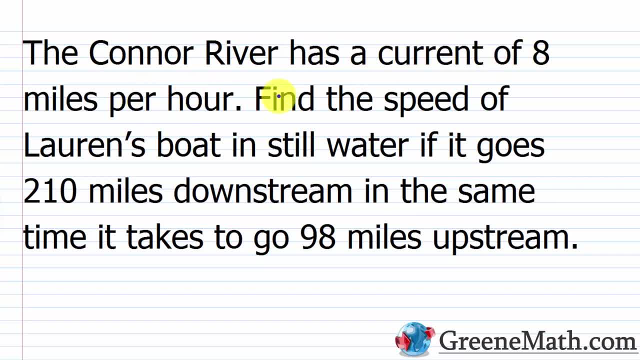 So the Connor River has a current of eight miles per hour. find the speed of Lauren's boat in still water if it goes 210 miles downstream in the same time it takes to go 98 miles upstream. Okay, So what are we being asked for? We're being asked to find the speed of Lauren's boat in still water. 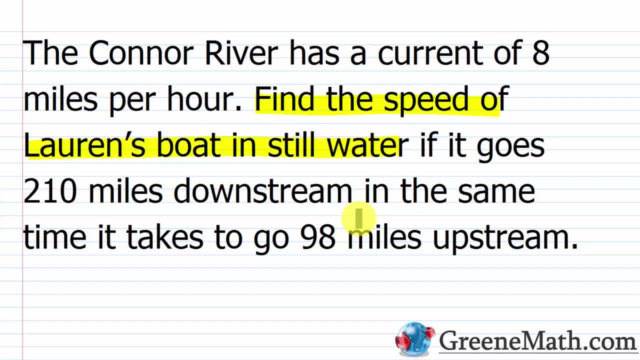 Okay, this is what we need to find. Now we're given a lot of time to figure out how to find the speed of Lauren's boat in still water. We have a lot of information to help us find this. It tells us the Connor River has a current. 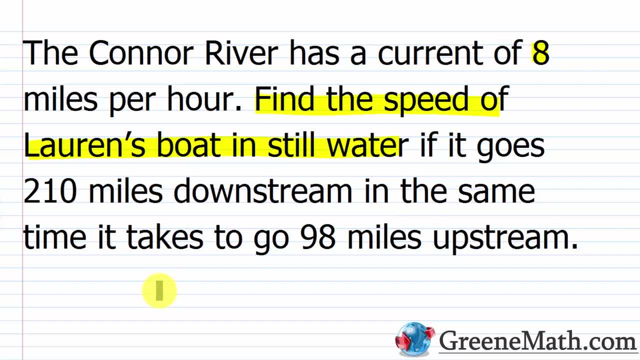 of eight miles per hour. It also tells us that her boat can go 210 miles downstream in the same time it takes to go 98 miles upstream. So when you get these type of problems, you need to understand the difference between still water upstream and downstream. Okay, so the way these problems work. 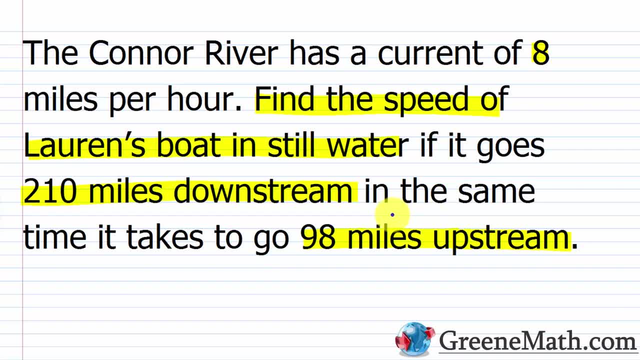 if you're in still water, basically there's no current. Okay, If you're going upstream, you are fighting the current. Okay, so you have to subtract the speed of the current away from the speed of the boat in still water. If you're going downstream, the current is pushing. 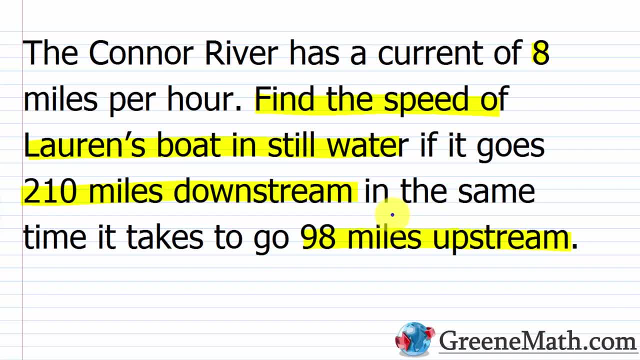 on you. Okay, so you're going with the current, And so now you need to add the speed of the current to the speed of the boat in still water. Okay, so we'll talk about that more in a second. For right now, our next step is to what It's to assign a variable to represent the unknown. 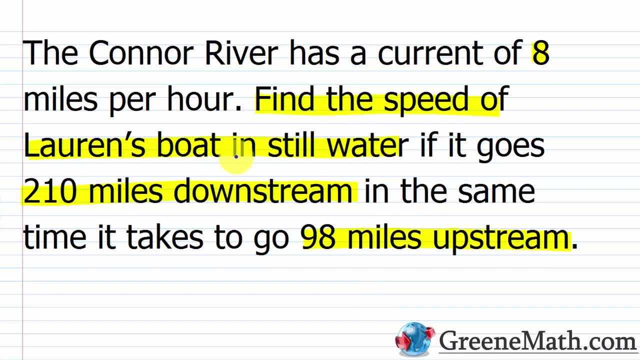 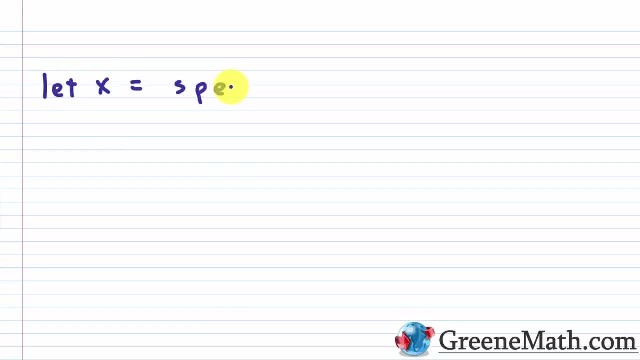 Our unknown here is the speed of Lauren's boat in still water, So I'm just going to let x be equal to that. So let's let x be equal to the speed of Lauren's boat in still water. Okay, so that's water with no current, All right, so let's take this down to. 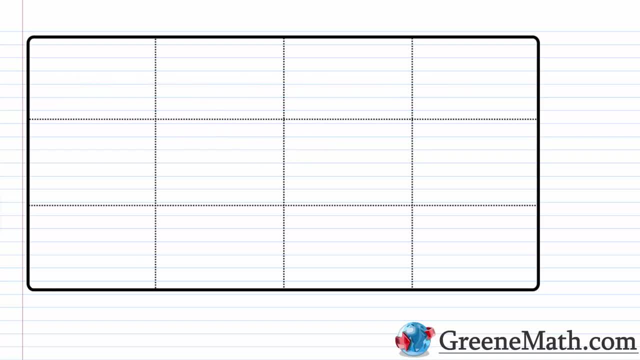 a little table so we can organize our information. So the first thing I'm going to do is put my distance formula up here Again. d stands for distance, And this is equal to r times, the speed of, which stands for rate of speed, multiplied by t, which stands for time travel. Okay, again. 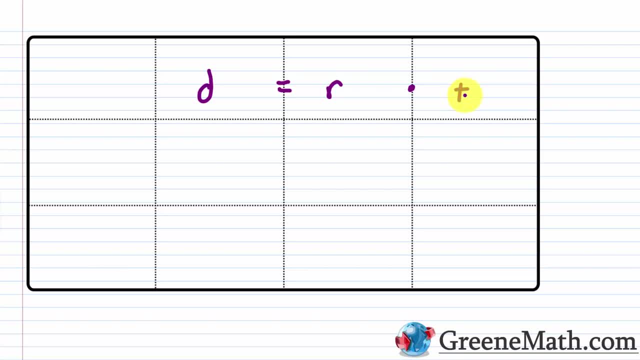 if I'm moving at 40 miles per hour and I do this for three hours, 40 times three is 120.. So I know it would go 120 miles. Okay, it's a very intuitive formula. So I'm just going to put my two scenarios. 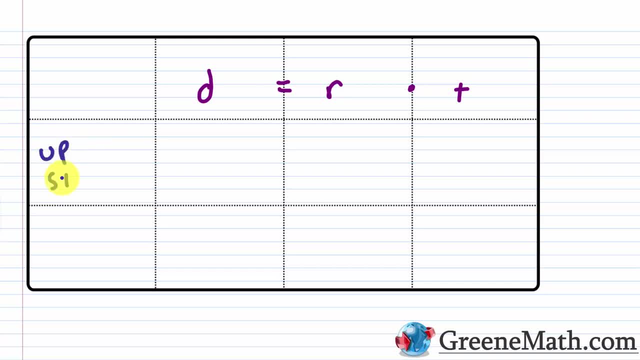 over here on the left. So we have upstream And we have downstream. So what am I told in the problem? Again, my rate in still water is unknown. That's what we're trying to find, But we expressed it as x, So I'm going to put x here, and I'm going to put x here Now. 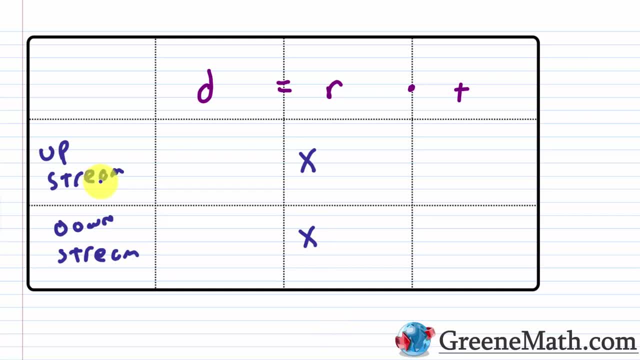 in the case where I'm going upstream, again I'm fighting the current. the current is eight miles per hour, So I've got to subtract eight away from the speed of the boat in still water, So I subtract eight away from x. In the case of going downstream, it's the opposite right: The current's pushing on. 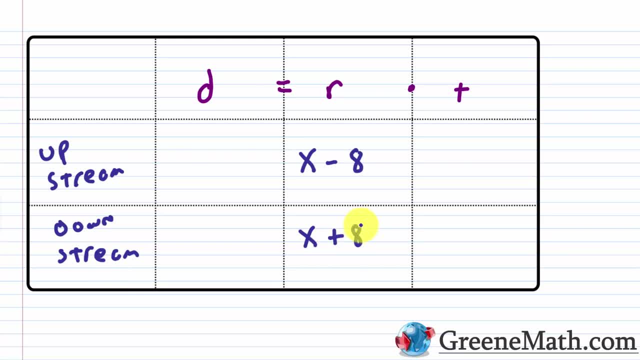 me, So I'm going to add eight. or again the speed of the current, So I'm going to add eight to the speed of the boat in still water. So for upstream, my rate is x minus eight. For downstream, my rate. 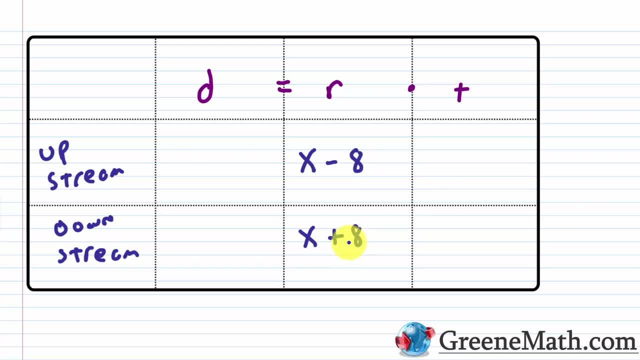 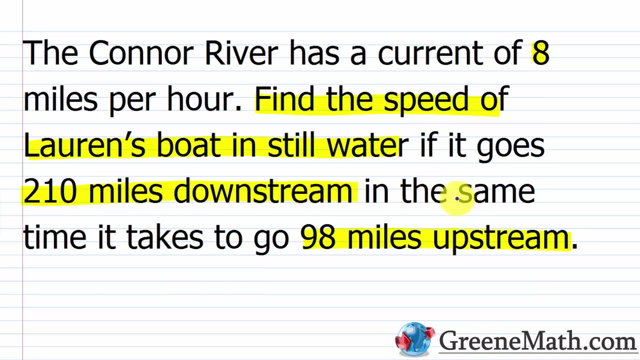 is x plus eight. Now what about the distance? Well, it specifically tells us that the boat goes 210 miles downstream in the same time it takes to go 98 miles upstream. So my distance for downstream will be 210. And my distance for upstream will be 98.. So for downstream, it's 210.. For upstream, 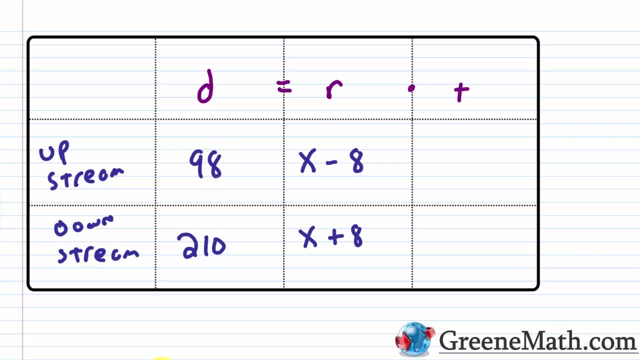 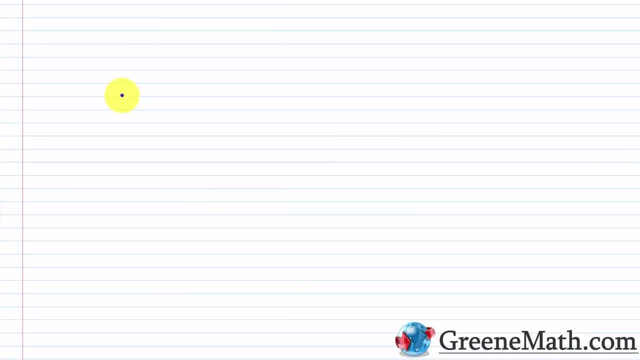 it's 98.. Okay, so now, what about the time? Well, to do the time, what we can do, we can solve the distance formula for time. So again, distance is equal to rate of speed, times, time travel. Okay, so if I divide both sides by r, what's multiplying t there? we know that this. 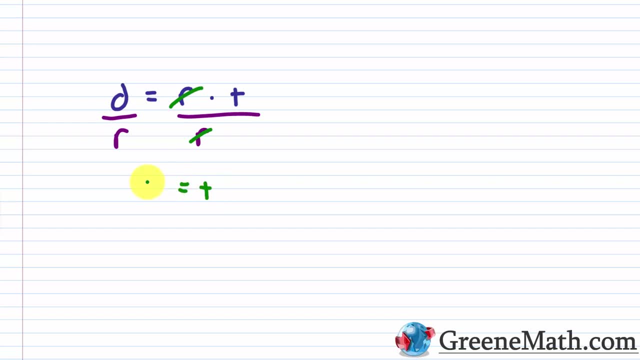 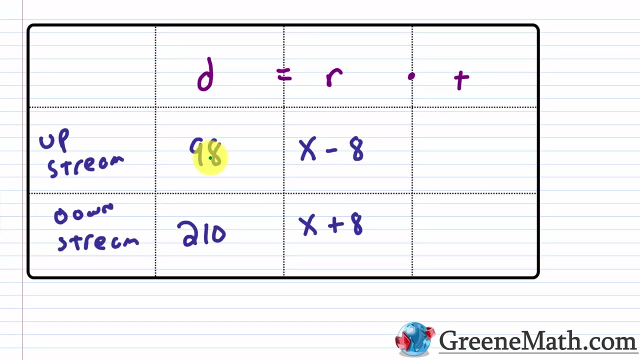 would cancel with this. I basically have that time is equal to distance over rate. So right now I have a distance and I have a rate for each scenario. So if I divide my distance by my rate, I'm going to have my time model. Okay, so let me erase this. So for upstream, my distance is 98.. 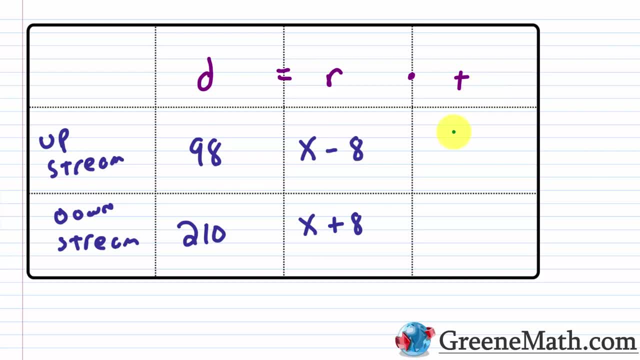 And my rate is x minus eight. So the time again is distance divided by rate. So it's going to be 98 divided by x minus eight. For downstream again, my distance is 210. And my rate is x plus eight. 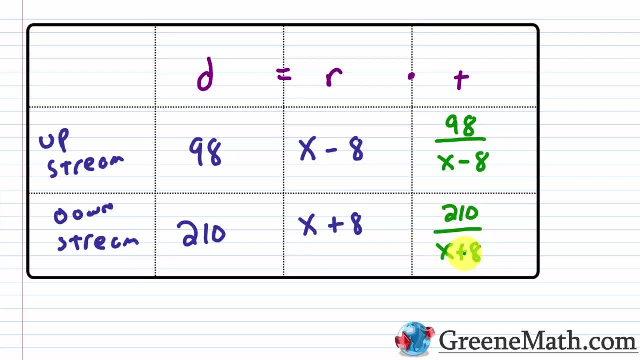 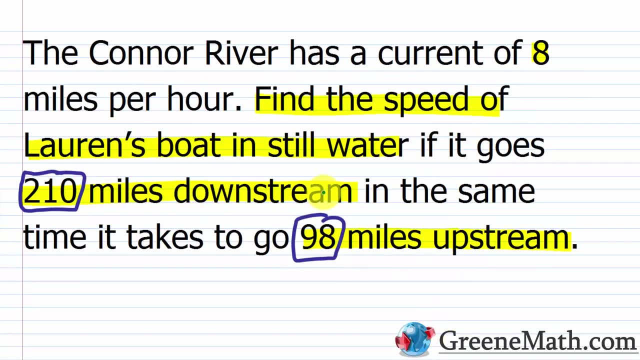 So my time for downstream will be 210 over x plus eight. Now it tells us in the problem- let me go back up- that the boat can go 210 miles downstream in the same time it takes to go 98 miles upstream. So 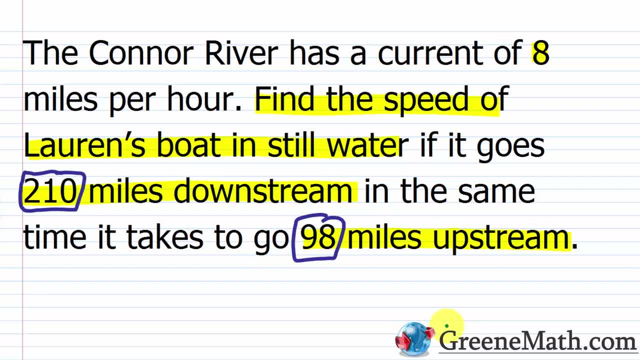 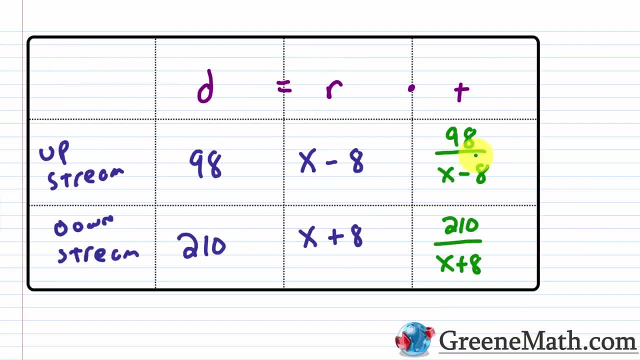 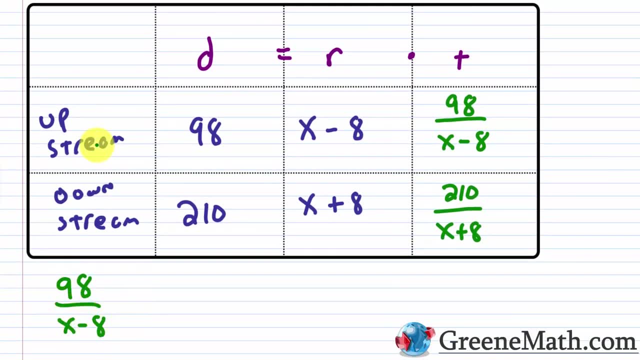 all we have to do is set the two times equal to each other, Because, again in the problem, it tells us that it's the same. it says in the same in the same time. Okay, So I can take 98 over x minus eight, So 98 over x minus eight. That's the time for going upstream and set this. 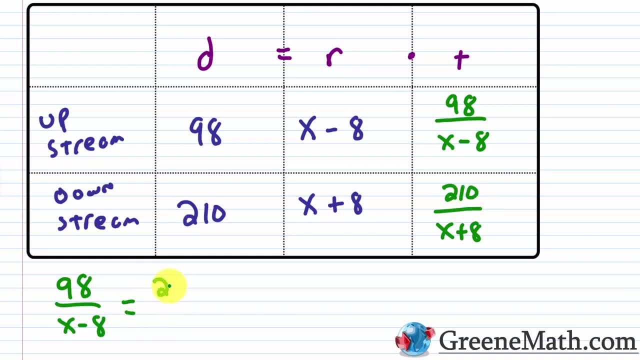 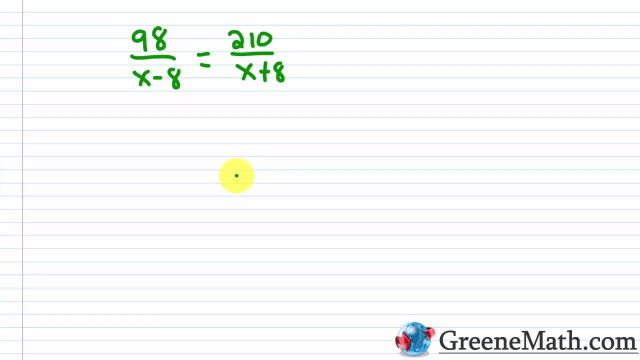 equal to my time for going downstream, which is 210.. So let me just copy this. we'll go to a fresh sheet. So how can we solve this? we already know how to solve rational equations. it's very, very easy. In this particular case, I don't need to. 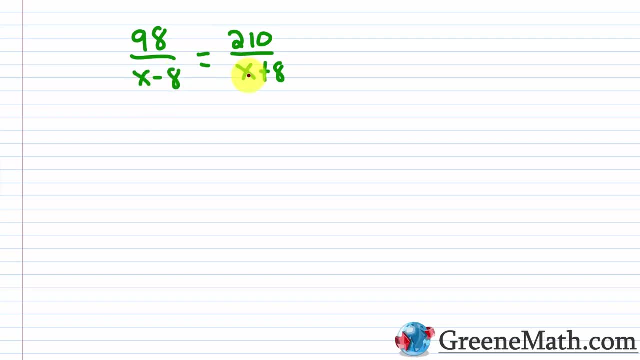 multiply both sides by the LCD. right the LCD would be x minus eight times x plus eight. I can multiply both sides by that, But a quicker method here would be just to cross multiply. So you take this guy right here, multiply by this. you take this guy right here, multiply by that. So essentially, 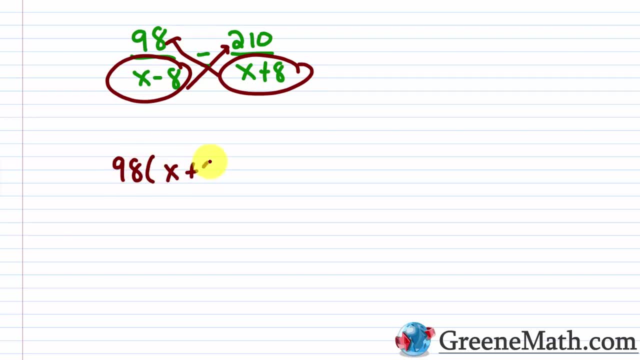 what I'd have is 98 times the quantity of x plus eight. So I can multiply both sides by that. So I could just start by using my distributive property on each side. But one thing you want to see here is that 98 and 210 are each divisible by 14.. Right, So to make this a little easier on myself, I'm going. 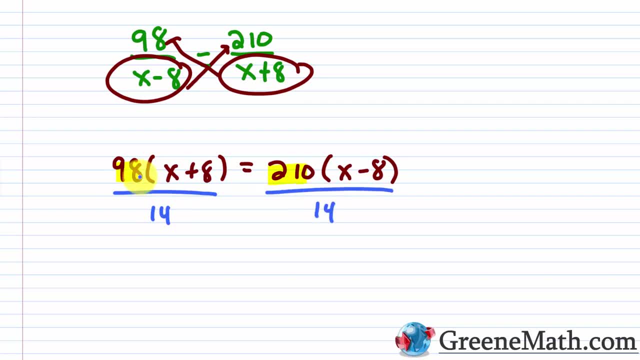 to divide both sides of the equation by 14.. Remember, this is multiplication here, So this is legal to cancel. 98 divided by 14 is equal to 90. So I'm going to divide both sides of the equation by 14 is going to give me seven, So I'd put a seven here. then 210 divided by 14 is going to give me. 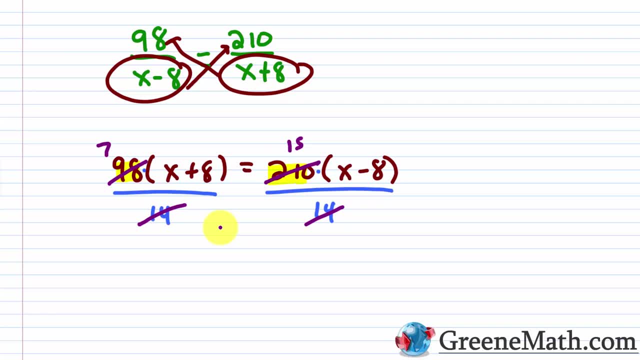 15.. And now I have smaller numbers to work with, So it's just going to make my life a lot easier. So seven times x is seven x, and then plus seven times eight is 56.. This equals 15 times x is 15x. 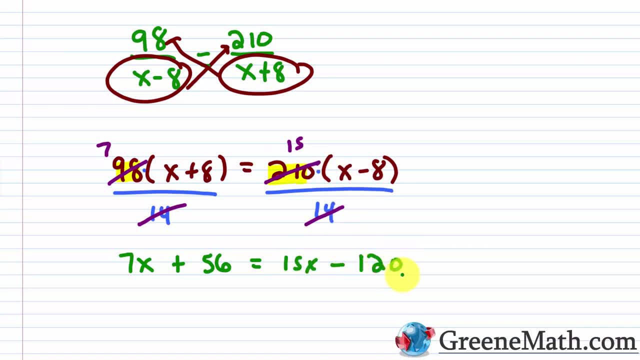 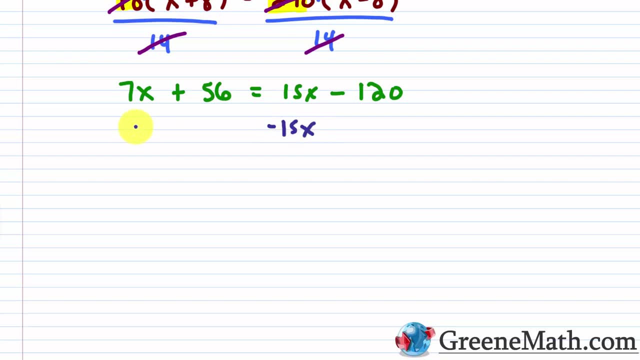 And then minus 15 times eight is 120. Okay, so let me scroll down a little bit, get some room going. Subtract 15x away from each side of the equation And I can subtract 56 away from each side of the. 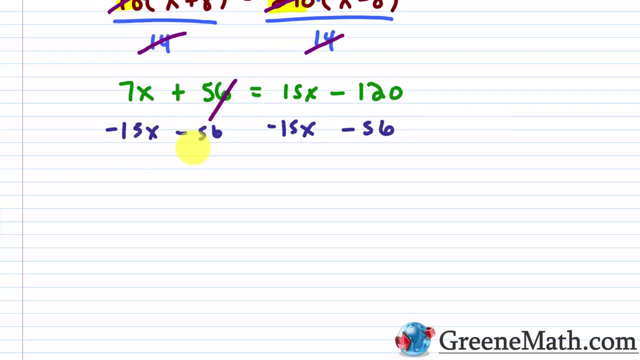 equation. So we know that this is going to cancel, and this is going to cancel. 7x minus 15x is going to give me negative 8x, And this will be equal to negative 120 minus 56 is negative 176.. If I finish, 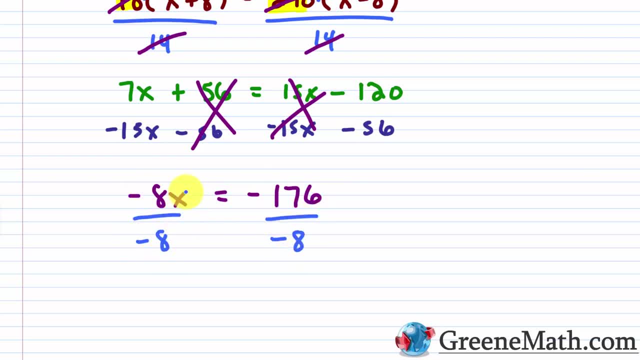 this up by dividing both sides by negative eight, right the coefficient of x there. what I'm going to get is this: cancels out. So I can subtract 15x away from each side of the equation And I can subtract with this. I'll have x is equal to 22.. So this is what we're looking for. I can't just put x equals. 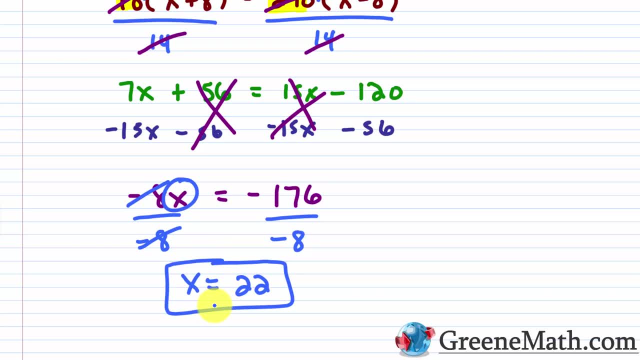 22.. Obviously, I've got to answer my question, But x tells me the speed of Lauren's boat, and still water, which is exactly what we want to know, right? So it's going to be 22 miles an hour. So. 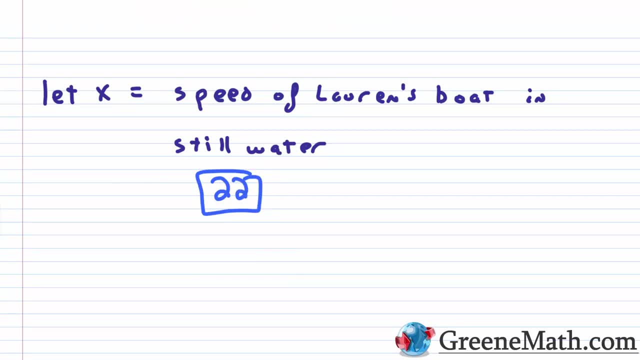 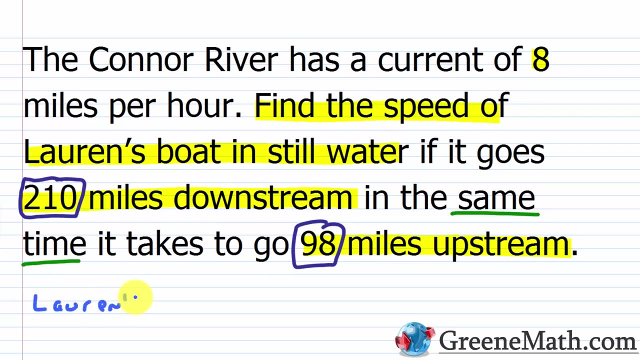 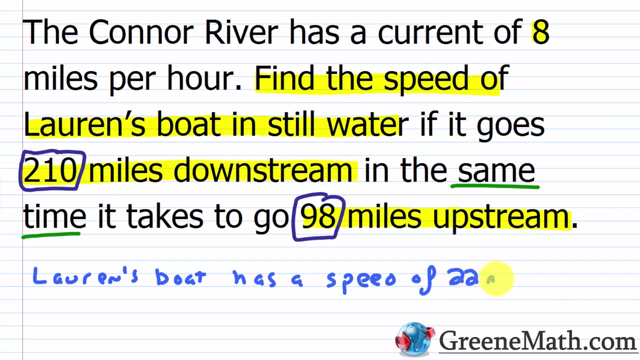 I can say: this is 22 here And let me go up and just answer my question. So I can just say that Lauren's boat has a speed- Let me make this better- Of 22 miles per hour in still water. So how can we check to? 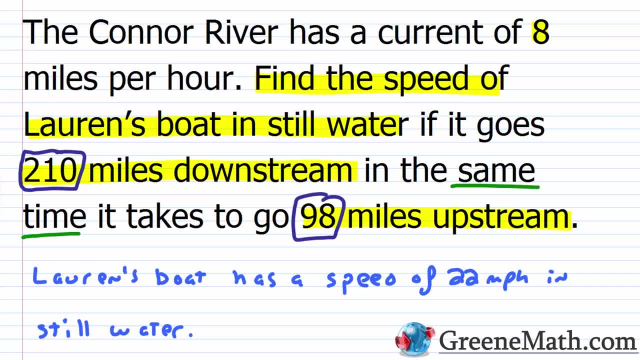 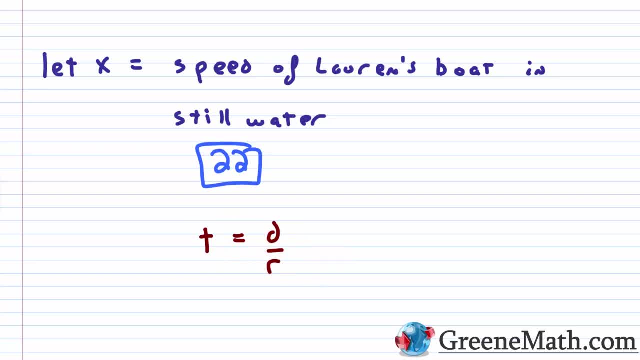 make sure we got the right answer. Well, again, if we go back to the fact that time is equal to distance over rate, we can just kind of think about the scenario we're getting here. So we're given for the downstream scenario. we know that her distance is 210 miles And we know that her 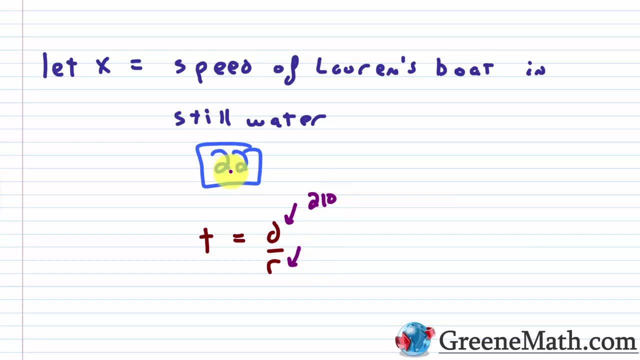 rate of speed is the speed of the boat and still water, which is 22,, plus the speed of the current, which is eight. So that's going to be 30. So 210 divided by 30 would be seven. So this is her. 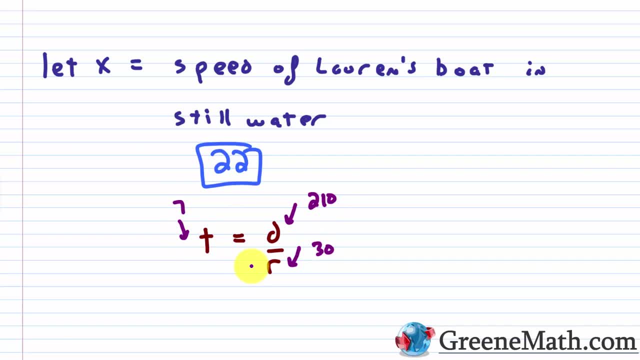 downstream scenario: it took her seven hours to go 210 miles. Now the other scenario. let me just set this up over here. We know that she goes 98 miles, Going at a rate of speed- Remember, if it's going upstream it's going to be 22,. the speed of the. 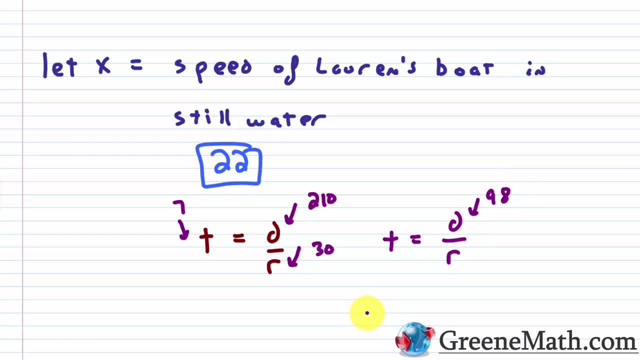 boat in still water, minus eight, okay, the speed of the current, which is going to be 14.. Okay, so this is 14.. And we know that 98 divided by 14 is seven. So this is true. right, It took her the. 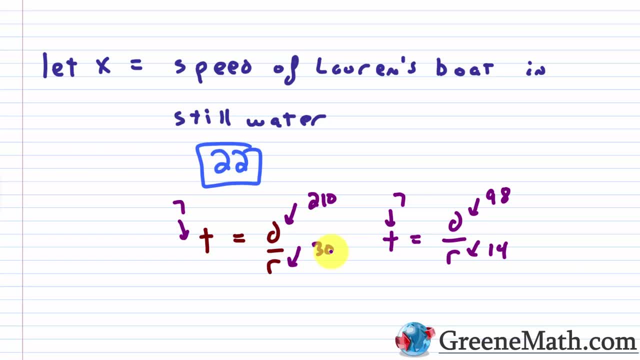 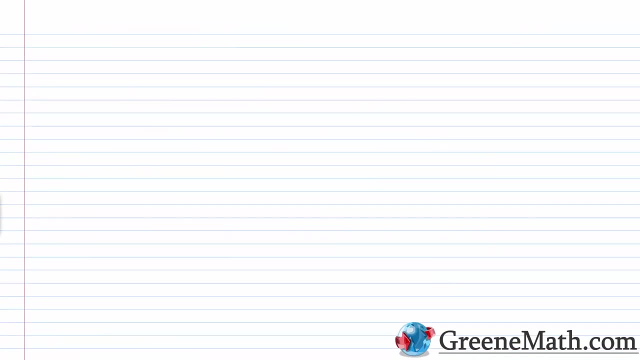 same amount of time to go 210 miles downstream- right Seven hours- that it takes to go 98 miles upstream- again seven hours. So our answer here is correct. Again, we can say that Lauren's boat is 22 miles per hour in still water. All right, now let's move on and talk about rate of work. 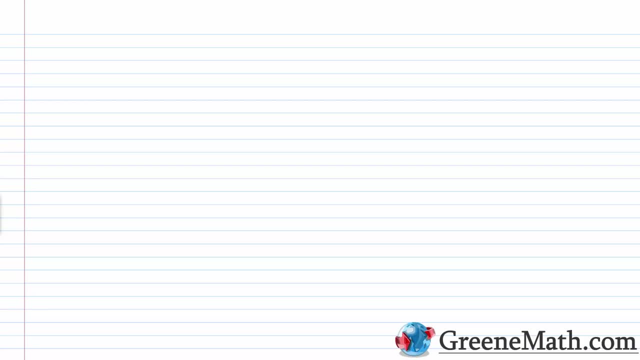 problems, otherwise known as work rate problems. So essentially, these are very easy problems to solve once you understand how to kind of set them up, And they just deal with the rate of speed at which a job can be completed, given the individual work rates from the people performing the job. 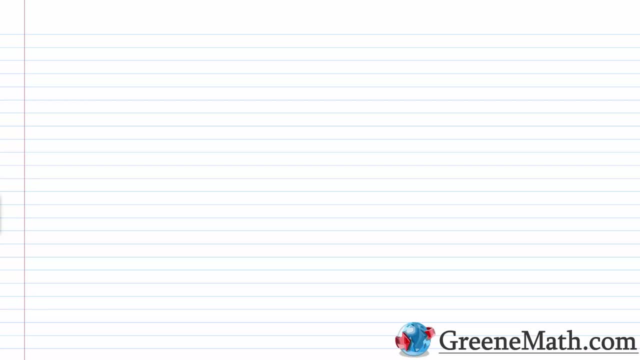 Okay, so again, very, very easy. If you understand the distance formula that we just used in the last video, you're going to understand this formula I'm going to give you here today. So the distance formula again is: D for distance is equal to the rate of speed, R times T for time travel. okay, Very, 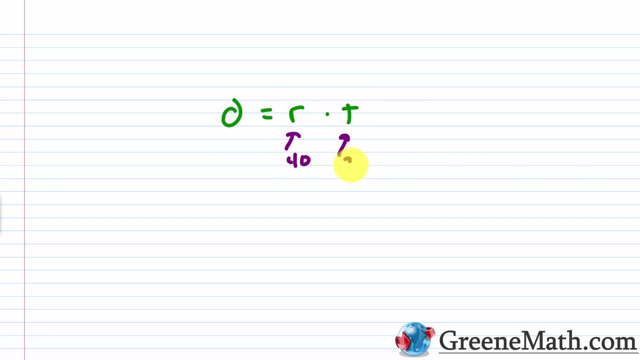 intuitive Again: if I go 40 miles per hour for three hours, 40 times three is what it's 120.. So I know I've gone 120 miles. okay, very intuitive, very easy to understand. The same thing goes when: 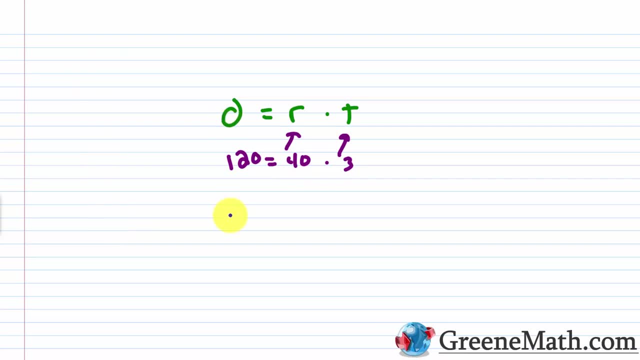 we work with work rate problems or rate of work problems. So instead of D, you have a, which stands for the amount of work completion, which I've got here, which is one job completed, And we think about this in terms of jobs completed. So it could be one jobs completed in pretty much every scenario that I've seen. But if you wanted to extend that and say, Okay, we have two jobs completed, 11 jobs completed, 2 million jobs completed, whatever, that is okay. but a here stands for the amount of work completed. This is equal to R, which is your rate at which the work is done. okay, otherwise known as a work rate. That's how these problems get their name. okay, then times T, which is our time, And that's the amount of time that your work is done. So D times T is the rate at which your work is done. right, so that's the amount of work that you're done. And this is another example that we use to calculate time travel. So you can see, here you can say t times the rate of work. So you can see, here you can say t times the rate of work. That's right, you. 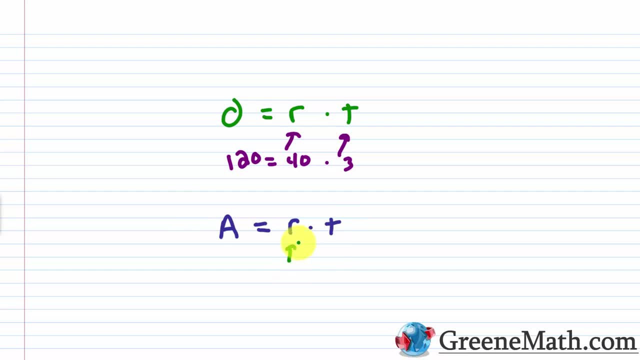 working for. So let's say, for example, my rate of work- and this will make more sense when I explain in a minute- is one over four. Okay, And I multiply this by a time of eight. What does that give me? We know that eight times one, fourth is two. So what does this mean? My work rate tells. 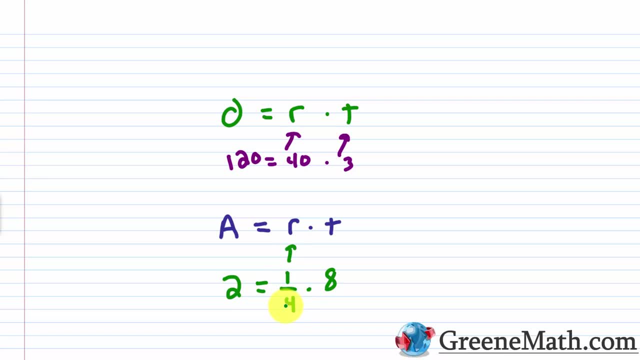 me how much of the job I can complete in one unit of time. So let's say, as an example, I'm working with hours. Let's say I was painting a house, So it takes me four hours to paint the house. Well, in one hour, one unit of time, I'm done with one fourth of that job. If I work at this, 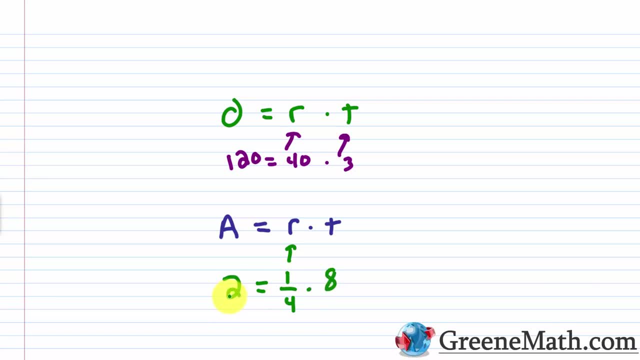 rate for eight hours. okay, I continue at eight hours. I'm going to paint two houses, right? Okay, that's all that same. If I change this to four, then this just becomes one, right? So if I work at a work rate of one fourth of the job per hour and I do this for four hours, well then I've got. 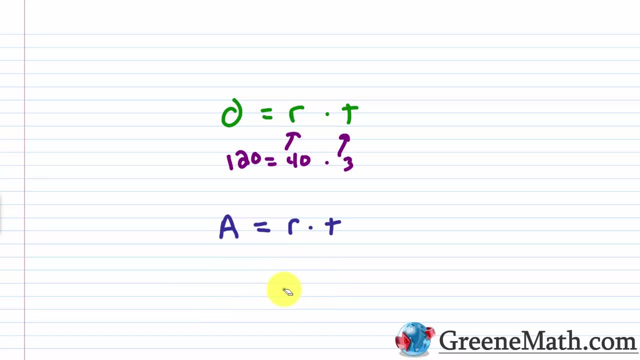 one completed job. Now, in almost every case, or in every case that I've ever seen, A is going to be one. So, basically, what you want to do is you want to paint two houses. So I'm going to paint two houses. So what you want to do is you want to paint two houses. Now, one of the things we want. 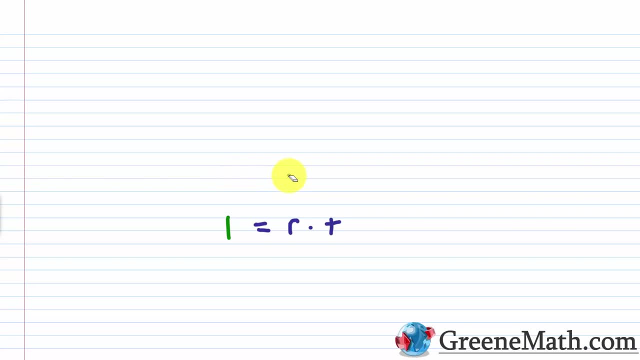 to focus on here and let me erase this. we don't need this information anymore. This R here is your rate of work, or your work rate. That's what you're focused on in the problem. So I'm going to divide both sides of the equation by T. That's what's multiplying R, So I can. 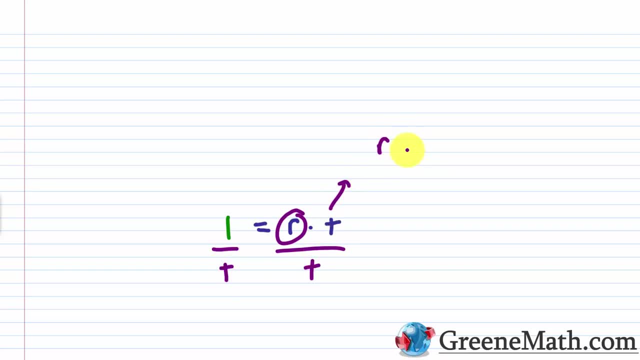 isolate, And I'll say that R, my work rate, or rate of work, is equal to one over T, So this is very important. You probably want to write that down in your notes if you're taking notes. This is what we're going to use in almost every scenario to get an answer. 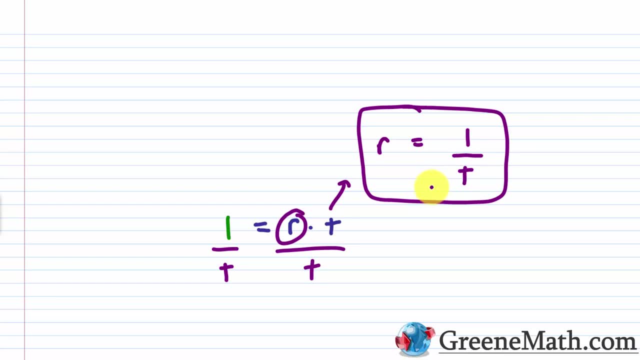 Okay. So you've got to know that if you're working on a problem like this and you want your work rate, just take a one and divide it by the amount of time it takes to complete the job. So again, in the case where we could paint the house in four hours while I would get a work, 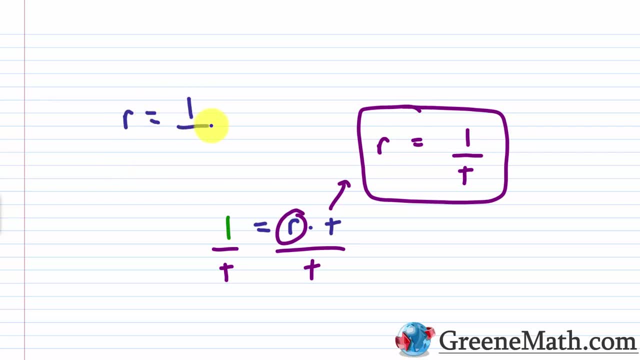 rate, my R would be equal to one over. takes four hours to complete it, So one over four. And all this is telling me is that in one unit of time, or one hour, I've completed one fourth of the job. Okay, As another example, suppose it takes me 15 minutes to wash my car- Okay. 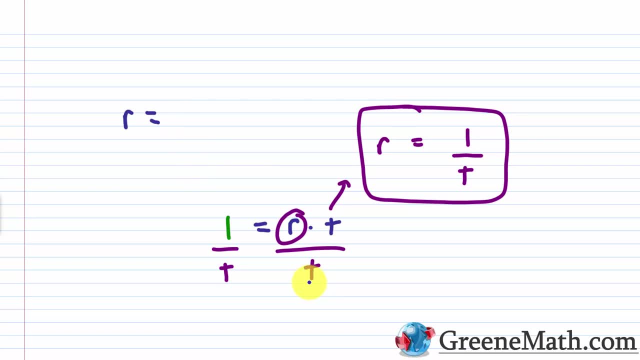 In one unit of time, which is now one minute because we're working with minutes. then I've done one over Again. it took me 15 minutes to complete it. So one over 15 or one fifteenth of that job is complete. Okay, So that's the general idea behind these problems. And now 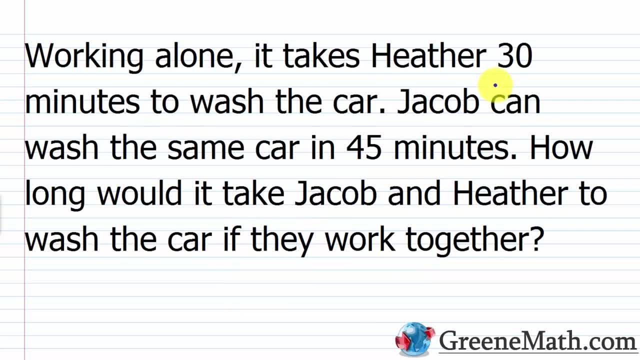 let's kind of jump in and look at one. All right, So working alone, it takes Heather 30 minutes to wash the car. Jacob can wash the same car in 45 minutes. How long would it take Jacob and Heather to wash the car if they work together? All right, So the first thing I'm going 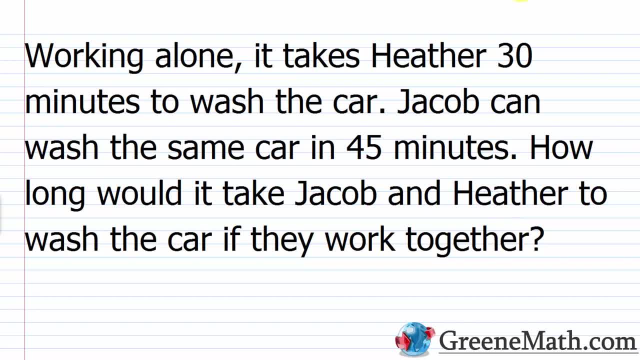 to do here, just like we always do, is just find out. what are they asking us to find? Well, the question we need to answer here is: how long would it take Jacob and Heather to wash the car? if they work together, This is a pretty typical scenario. So you have their 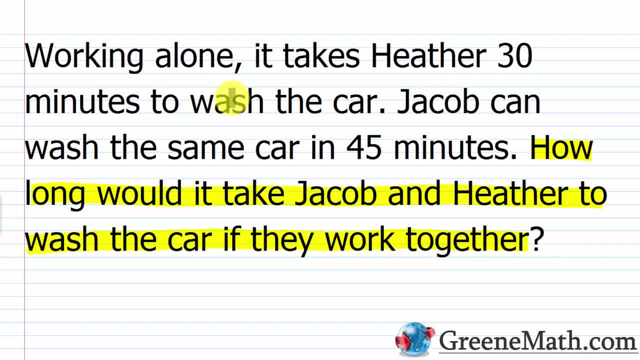 individual rates of work. right, We know that Heather takes 30 minutes to wash the car. We know that Jacob takes 45 minutes to wash the car. But hey, if they work together at the same speed, they're going to wash the car in 45 minutes. So we're going to have to find out. 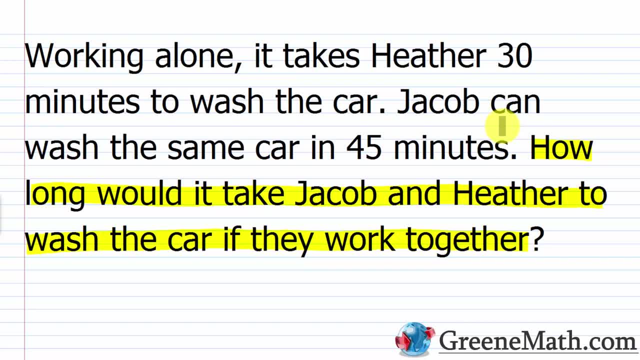 that they're working at. when they do it individually, how long would it take for them to wash the car? Okay, So that's what we're trying to figure out. So what I'm going to do is I'm going to let a variable like X be equal to that. So I'm going to go to the next page and 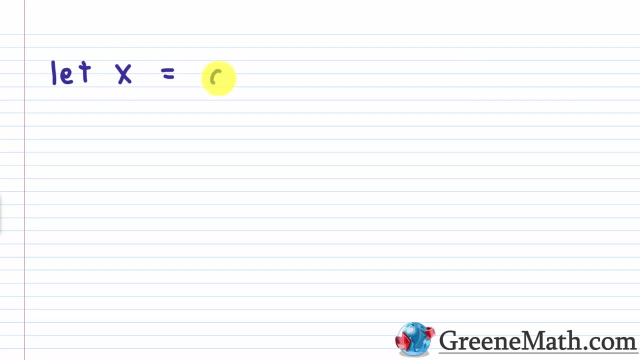 I'm just going to say that we're going to let X be equal to the amount of time And I'm just going to say to complete the job, to complete the job, Right. But if you wanted to be more detailed, you could say the amount of time to. 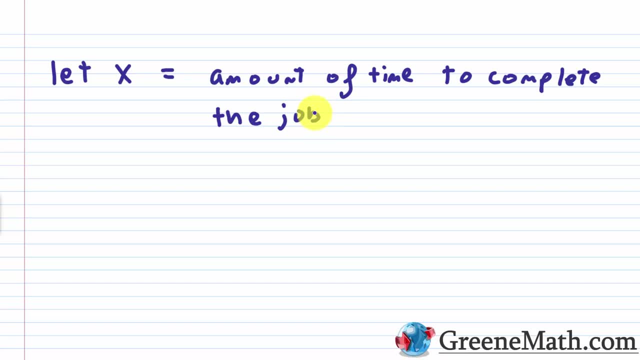 complete the job When Jacob and Heather work together. Okay, And of course, since we're working with minutes here, the units are going to be minutes, Okay. So you got to make sure of that because, since some of these problems, you have crossovers between minutes and hours. 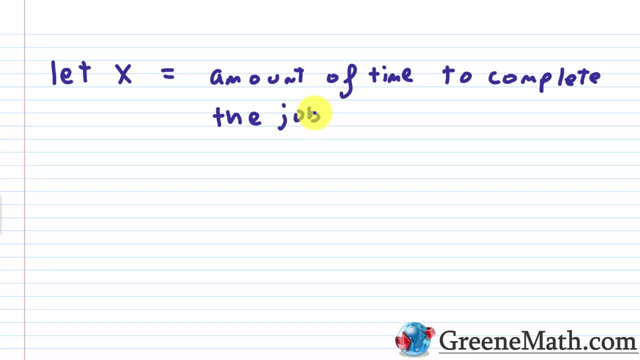 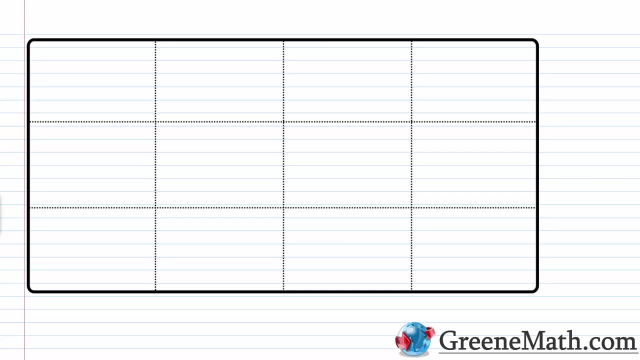 you can have minutes and seconds, you know, so on and so forth, But for this one it's very easy. We're just working with minutes, All right. So let's go down to a little table and we're going to organize some information And then, once you see this, in the next few problems you're going. 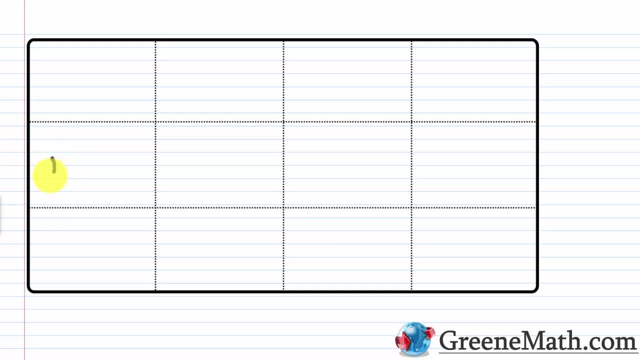 to go right through it. Okay, Very, very simple. So of course, we have Jacob and we have Heather. Now the first thing I'm going to write is the rate of work. So the rate of work- And before we started this problem we talked about how to get it- It's one over. 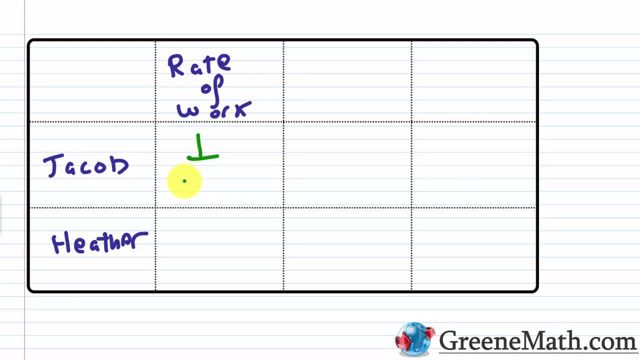 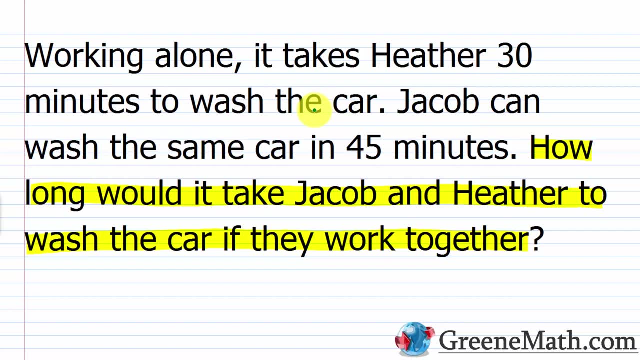 the amount of time they take to complete the job. So I'm going to put a one over and then blank for each one. Let's go back up. So for Heather it takes 30 minutes to wash the car, So her rate of work would be one over 30. Again, for every minute that passes she's done one 30th of that. 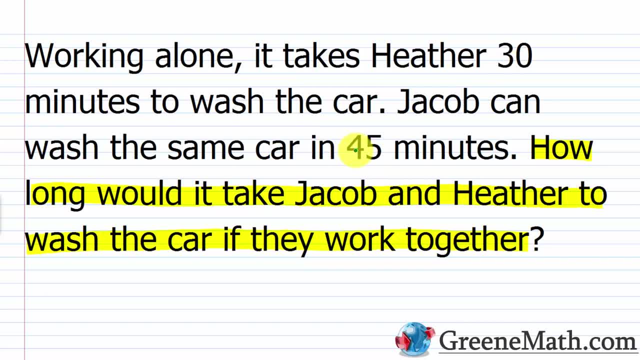 job For Jacob. his is going to be one. It takes him 45 minutes to wash the car, So it's going to be one over 45. Every minute that passes he's going to be done with one over 45, or one 45th of that. 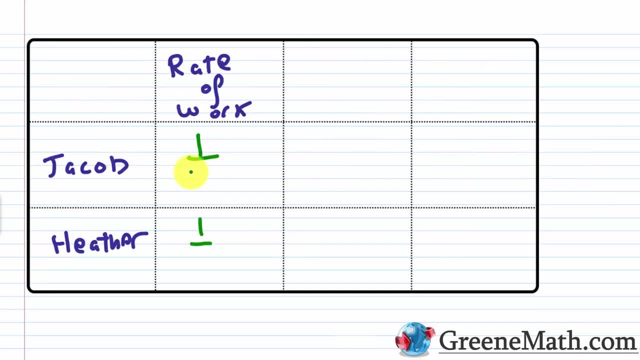 job. So let's go down again. for Jacob, He's got a work rate of one over 45. for Heather, She's got a work rate of one over 30.. Okay, So now I'm going to put time working together. So time working. 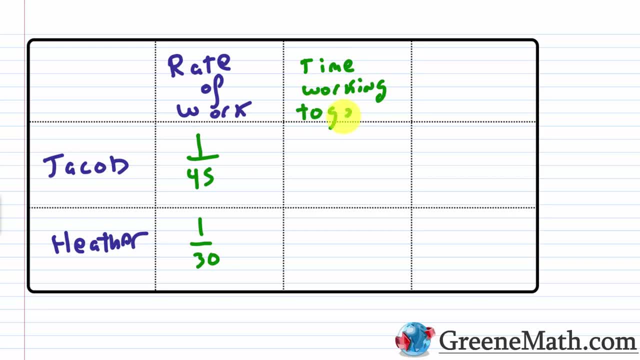 and then together. Now we modeled this on the page, Okay. So I'm going to put this as X here and X here. Okay, It's the same in each case. Now the next thing you need is the total contribution of each person. How much of the car does Jacob? 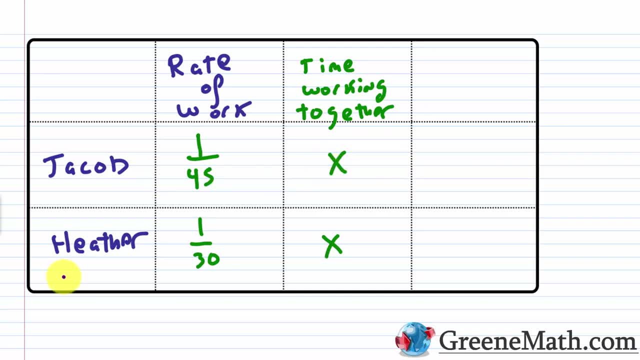 get done in this amount of time? How much of the car does Heather get done in this amount of time? So I'm just going to write this as total contribution. Okay, So to get this we can just multiply, right, Because if you want to know, 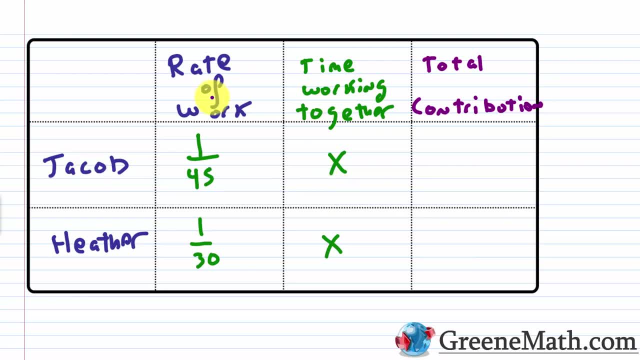 the amount of work that Jacob performed. I just multiply my R times my T right My A. the amount of work that's performed is R the rate of work times T the time that you're doing that work for. Well, I've got my rate of work, I've got my time that I'm working for. So my contribution. 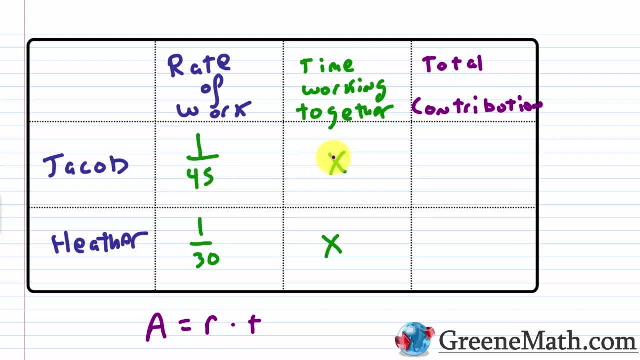 here, or the amount of work that's being performed for Jacob is one over 45 times X. You could write it as one over 45 times X, or you could write it as X over 45, which is probably a little better. Same thing goes for Heather. It's going to be. 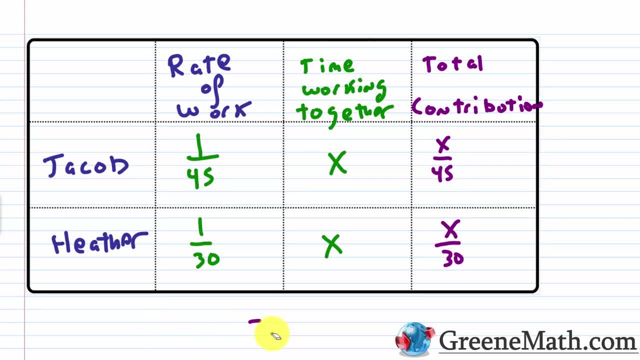 X over 30,. right, Just multiply across Very, very easy. And now what we need to understand is that between Jacob and Heather, they're going to complete one job. Okay, So the equation here is very easy to set up: Jacob's contribution, which is X over 45,, plus Heather's contribution. 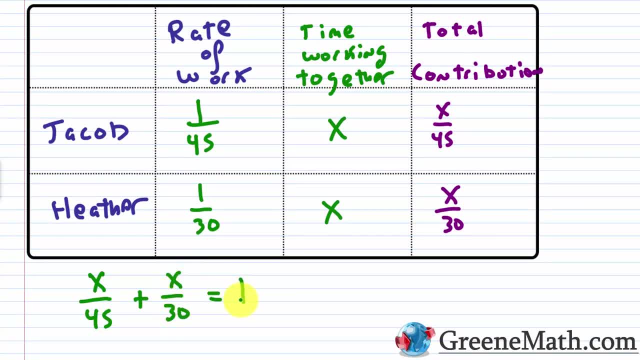 which is X over 30, is going to be equal to one. Again, that's for one completed job. So the first time you see this it might not make a whole lot of sense. But again, after you solve like two or three of these, you're going to find that these are the easiest problems. 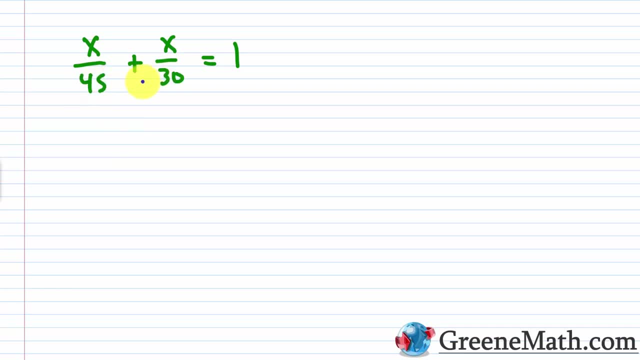 to solve. So let's copy this. So what I'm going to do to clear these denominators, I'm going to multiply both sides of the equation by the LCD. The LCD: if I look at the denominators, I've got 45 and 30, it's going to be 90. So I'm going to use my distributive property here 90 times X. 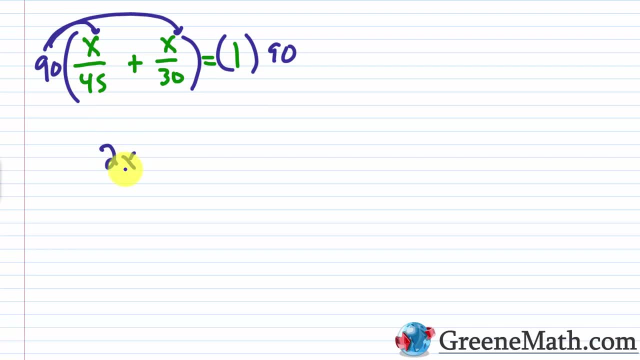 over 45,. 90 divided by 45 is two. two times X is two X. Then plus 90 divided by 30 is going to be three. then times X is three X And this equals 90.. Sum on the left so two X plus three X. If I. 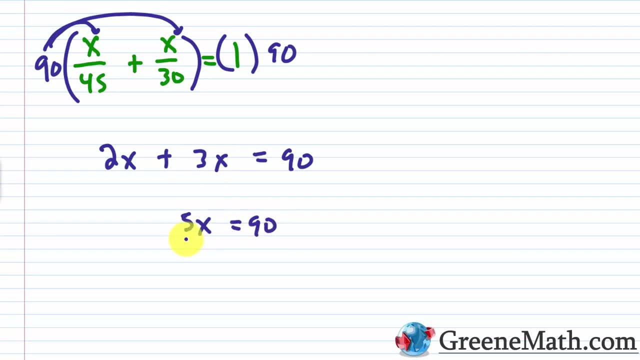 combine like terms there, I get five X. This equals 90. Divide both sides of the equation by five And we're going to find that X is going to be equal to 18.. So 18 is the number of minutes that they each have to work when they're working. 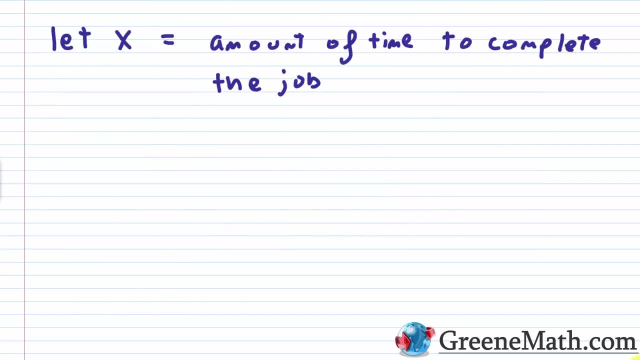 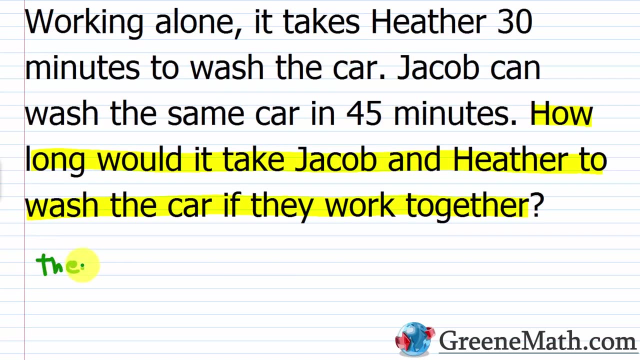 together to complete the job, right? So if we go back up again, we said amount of time to complete the job, that's when they're working together And of course, this is in minutes. So let me just say that they work for 18 minutes. 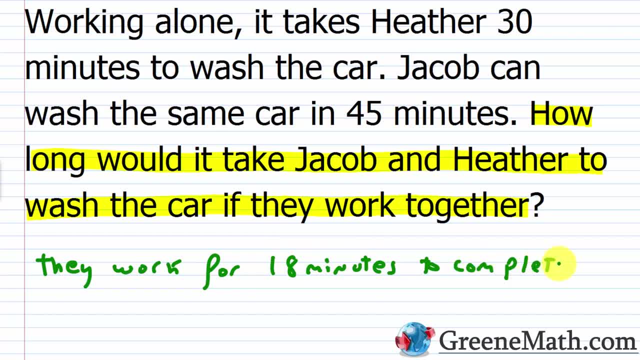 18 minutes to complete the job. okay, You can answer a whole lot of different ways there. That's just a very simple sentence to say they work for 18 minutes to complete the job. Now is it correct? How can we check this? Well, we can take the fractional amount that Heather does and the 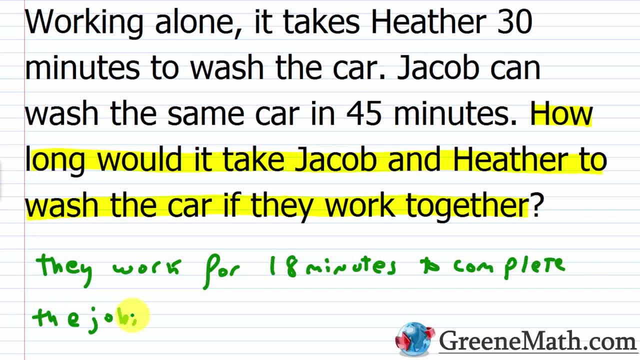 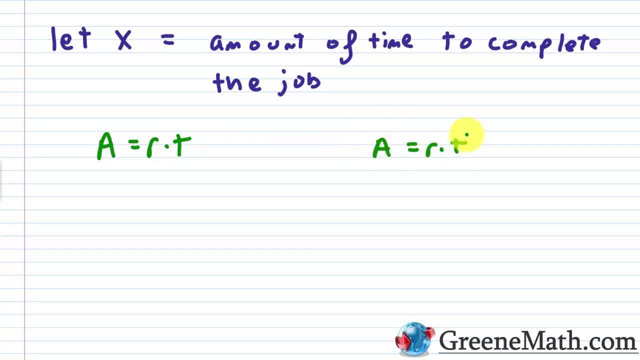 fractional amount that Jacob does and add those together and see if it equals one. So we know that if we go back down, A is equal to R times T. I'm going to put two scenarios. A equals R times T, So how much or what amount of the job does Heather do? Well, remember her R. her rate of work is 1. 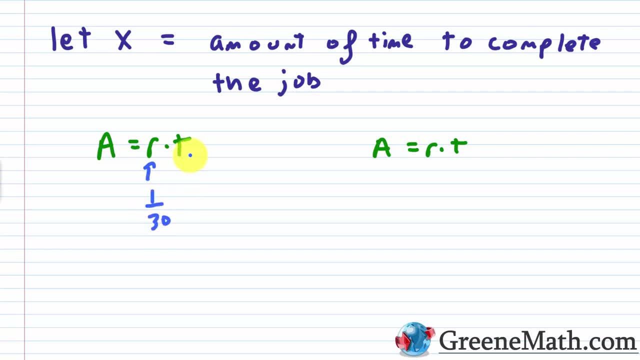 over 30. And she works for T minutes. And again we found that the time that they're going to work together, which we labeled as X, was going to be 18.. So essentially, I'm going to put this as times. 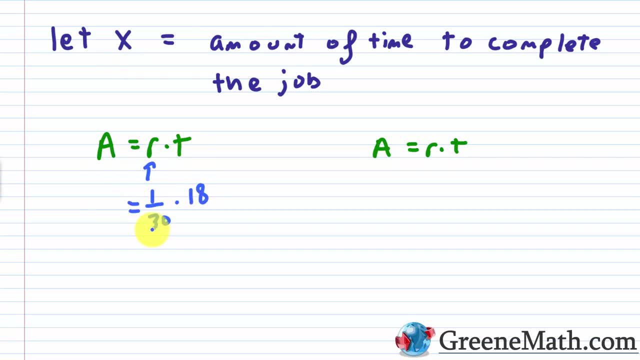 18.. That's going to give me the amount of work that she does. So between 18 and 30,, I have a common factor of 6.. So if I divide 18 by 6, I get 3.. If I divide 30 by 6,, 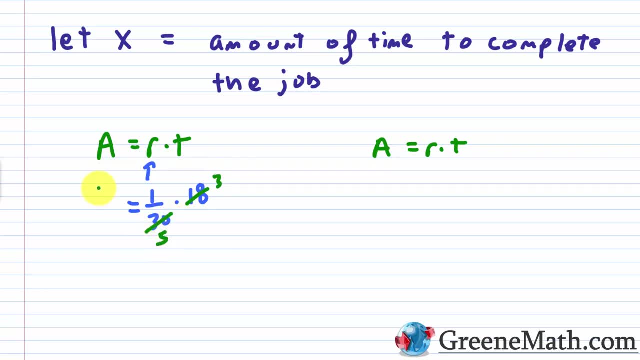 I get 5.. So I get three-fifths there. So this is going to be three-fifths. That's the amount of work that she completes. Now for Jacob. he's a little bit slower, So his rate of work is 1 over. 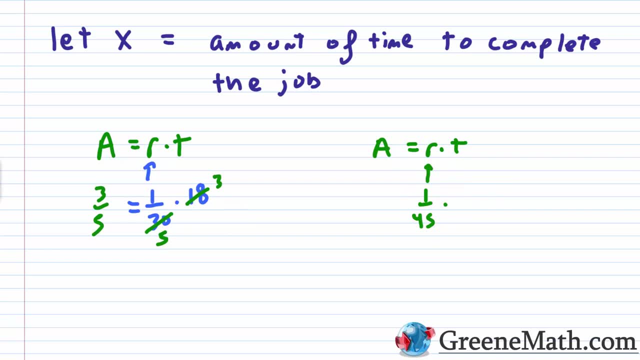 45. And the time is the same right, Because they work the same amount of time when they're working together. So this is 18.. Each here is divisible by 9.. 45 divided by 9 would be 5.. 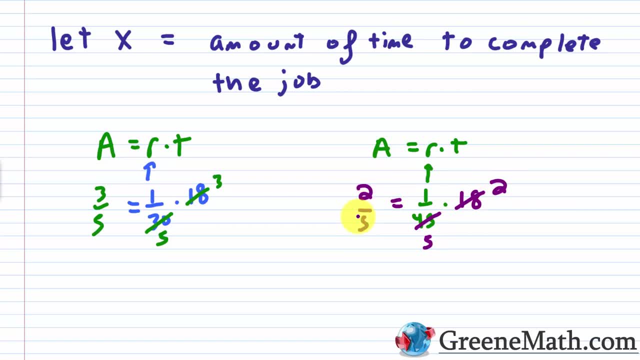 18 divided by 9 would be 2.. So this is two-fifths. Now, if you go ahead and take the amount of work that Jacob completes, which is two-fifths, That's what he does in 18 minutes And you add: 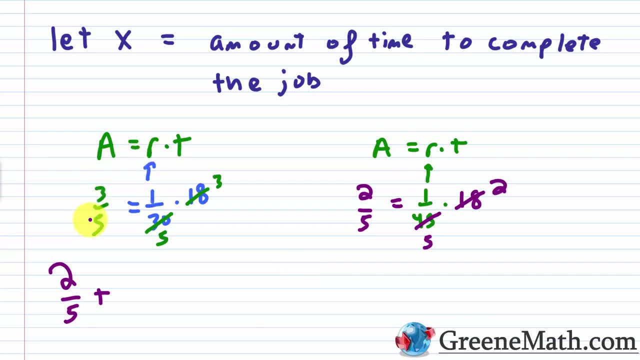 that to the amount of work that Heather completes, She's got three-fifths of the job that's completed And that's what she does. in 18 minutes. You do get 1, right: Two-fifths plus three-fifths. 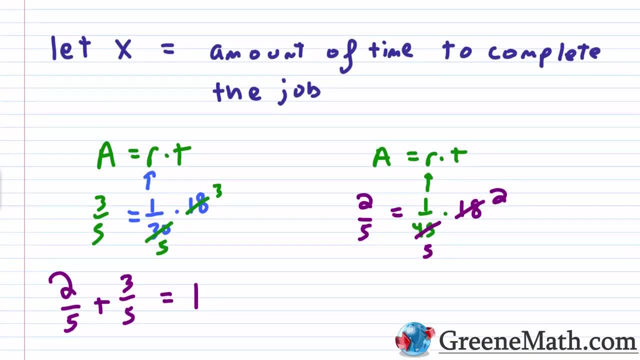 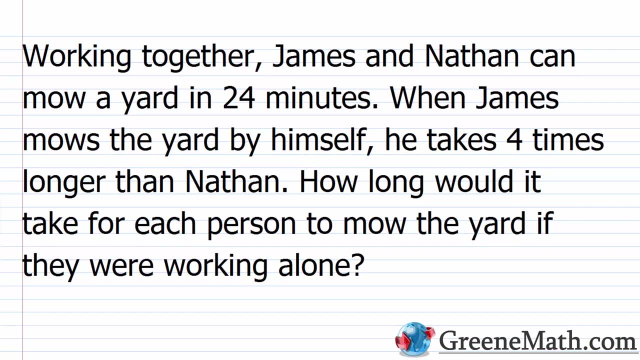 is five-fifths, Five-fifths is 1.. So we can say our answer here is correct. They work for 18 minutes to complete the job. All right, Very easy overall. Let's take a look at another one. So, working together, James and Nathan can mow a yard in 24 minutes. 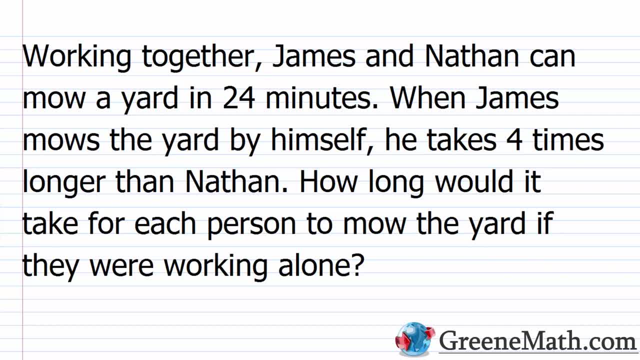 When James mows the yard by himself, he takes four times longer than Nathan. How long would it take for each person to mow the yard if they were working alone? So in the last problem, we knew their individual rates of work, right, We knew that. 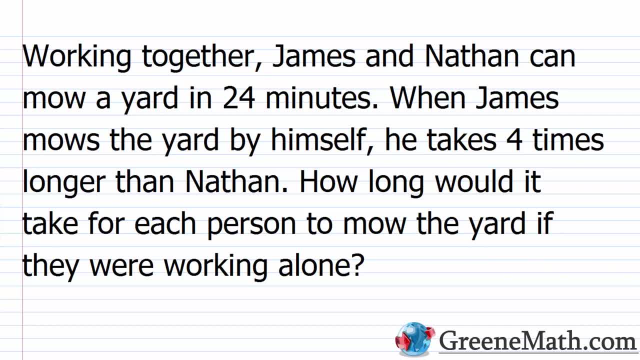 for Jacob, he could wash the car in 45 minutes. For Heather, she could wash the car in 30 minutes. But we didn't know, or we could say we had defined, how long it would take if they worked together In this case. we know how long it takes when they work together, right? It tells us right here. 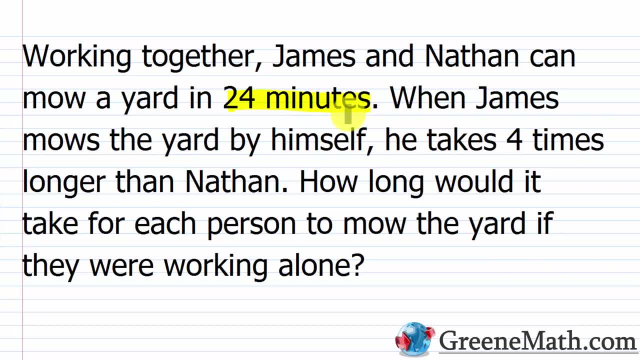 24 minutes, But we don't know how long it takes them individually, Okay. So that's the question here: How long would it take for each person to mow the yard if they were working alone? So how long does it take for James? How long does it take for Nathan? 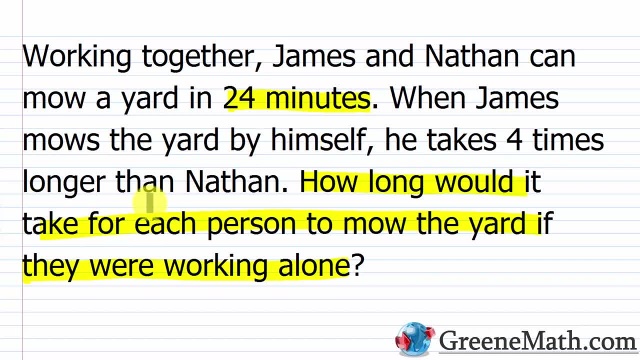 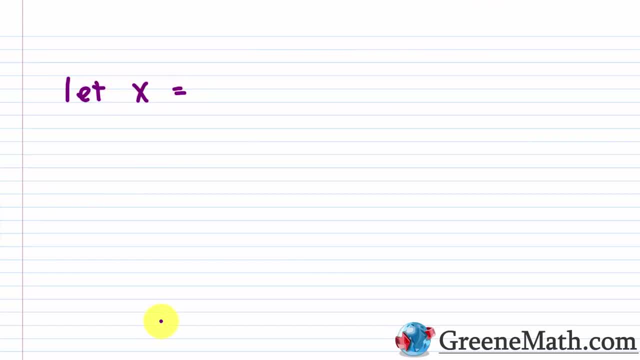 So we're specifically told that James takes four times longer than Nathan. So let's let X be equal to the amount of time it takes for Nathan to mow the yard by himself. So the time for Nathan, and I'm not going to write the rest. You can write the rest if you want, but it's just the. 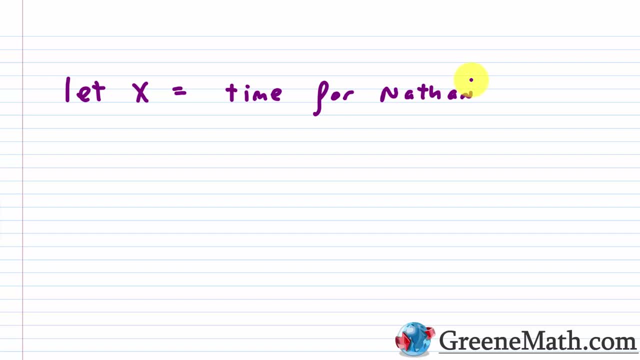 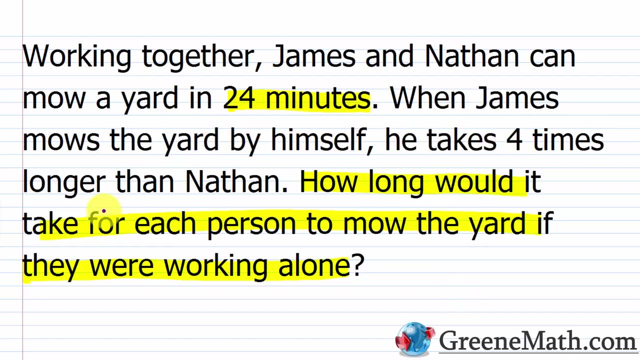 time for Nathan to mow the yard by himself. So the time for Nathan to mow the yard by himself. So then, because James takes four times longer? again, it tells us that right here. when James mows the yard by himself, he takes four times longer than Nathan. 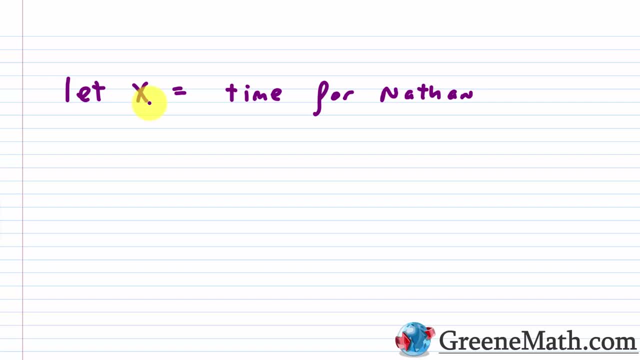 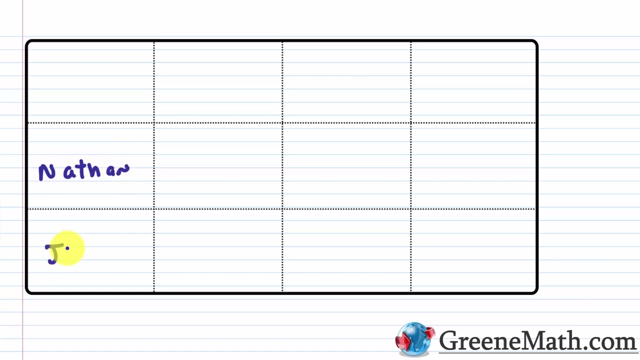 What I can do is just multiply four times X to get the time for James. So I could say then four X is equal to the time for James. Okay, Let's go back to our table and kind of organize this. So again we have Nathan and James. So we have Nathan and we have James, And again. 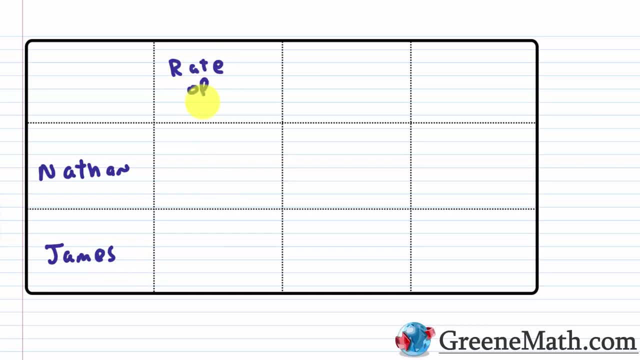 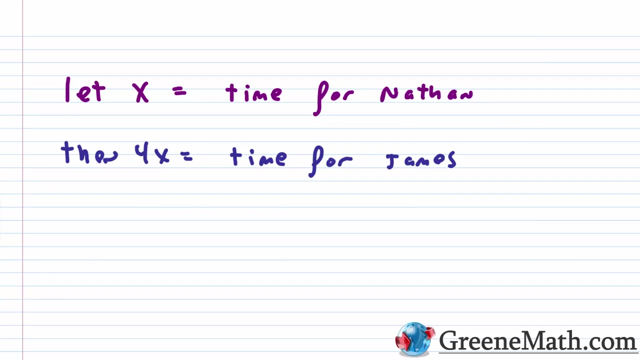 we have the rate of work, the rate of work and we have the time working together And then we have their total contribution. So for the rate of work, remember it's one over the amount of time it takes for that person to 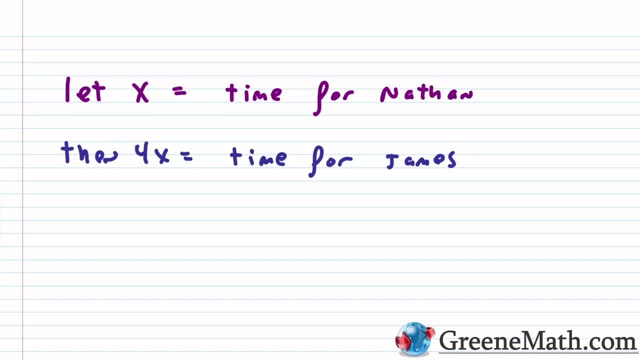 complete the job. So if it takes me four hours to paint a house again, the rate of work is one over four. That's how much I'm going to do in one unit of time. So in an hour I'm going to do one fourth of the job. Here we know. for Nathan, this is in terms of minutes. 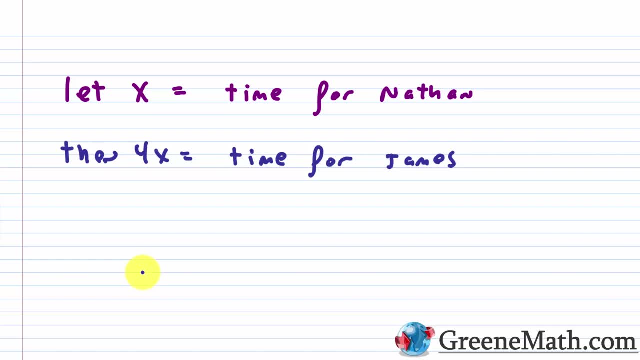 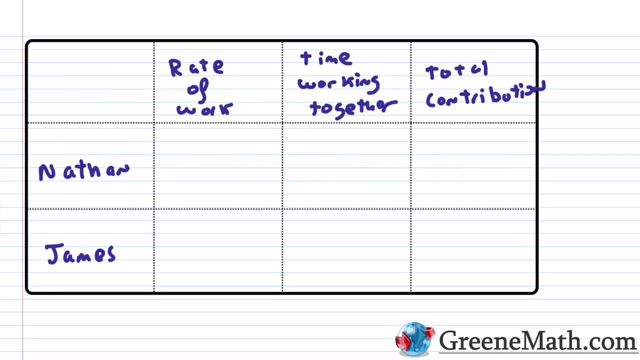 he can complete one over X amount of that job every minute. Okay, So for James it's going to be one over four X every minute. So for Nathan it's one over X. For James it's one over four X The time working together. it tells us that in the problem It 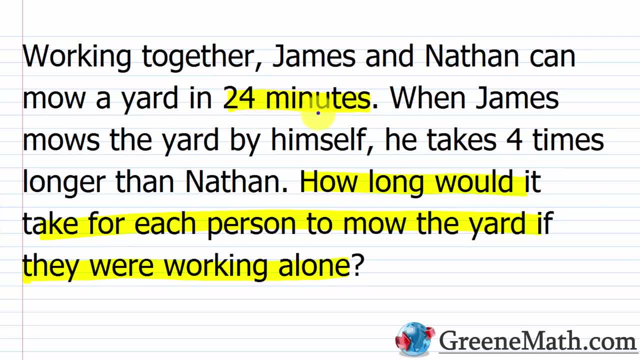 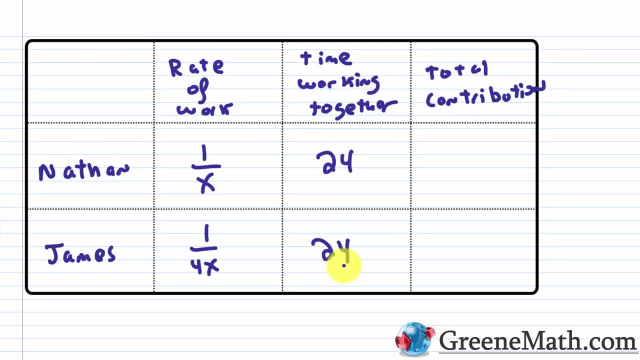 tells us specifically that James and Nathan can mow a yard in 24 minutes. That's again when they're working together. So each person is going to work for 24 minutes in this scenario. So what's their contribution? Again, you just multiply. This is the rate of work, This is the 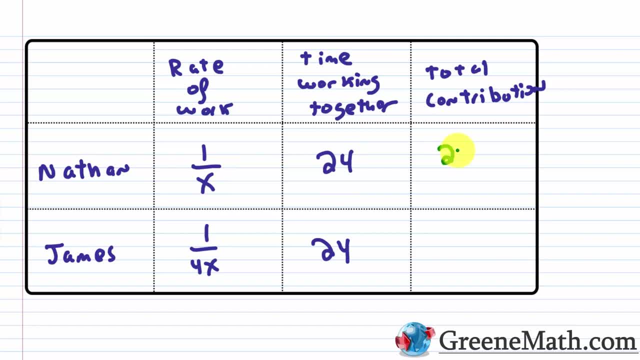 time working. So 24 times one over X. You can do just 24 over X to make it simpler. And then here it's 24 over four, X, which we could simplify. 24 over four is six, So I could just say this is six over X. Now how do we get an equation? 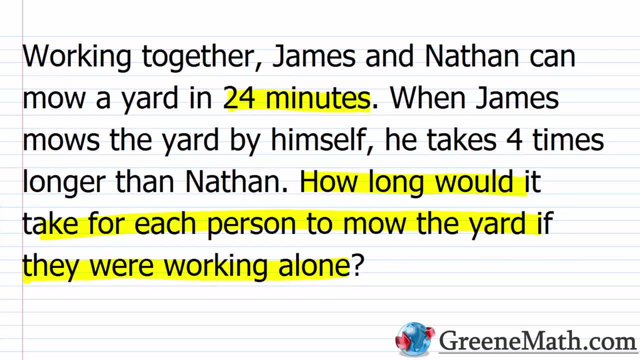 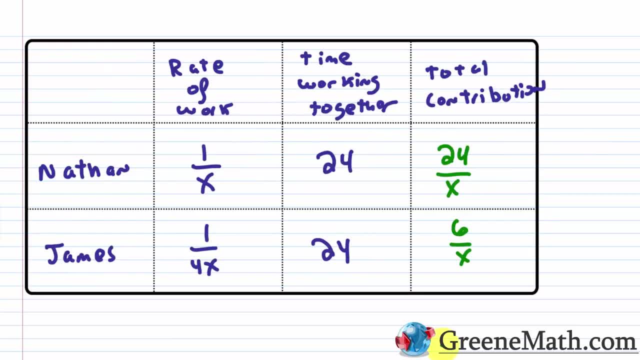 going Well. we know that when we sum the amount of work done from both of them over this again 24 minute period, they've completed one job. So the amount of work that Nathan does is 24 over X. Okay. 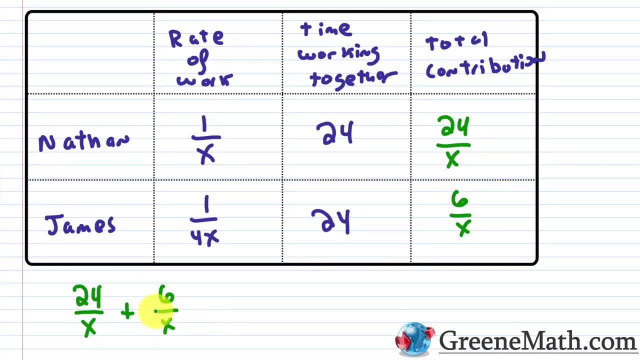 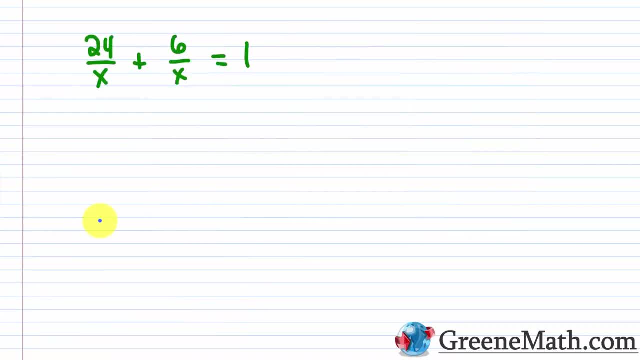 So the amount of work that James does is six over X. If I add these two amounts together, I should get one completed job. So let's copy this, All right. So what can I do here? Well, I can multiply both sides of the equation by X. right, That would be the LCD. So I'll multiply. 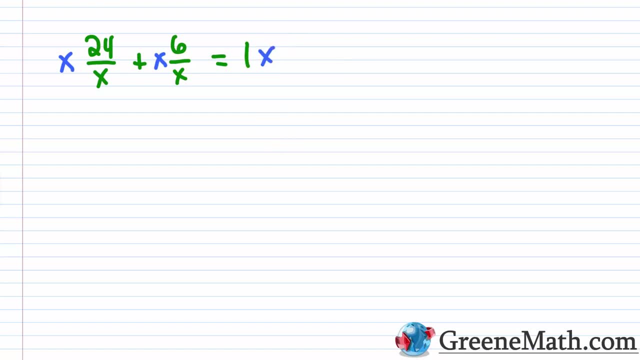 this by X, this by X and this by X. So essentially, this is going to cancel, This is going to cancel. You'll basically just have what: 24 plus six, which is 30, is equal to X. So that's really a piece of cake. We've immediately found that. 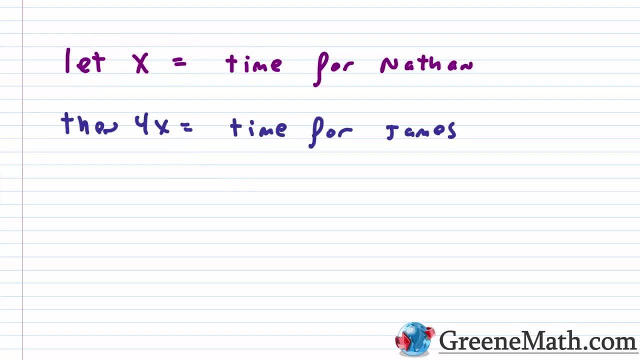 X is 30. And we know that X was the time for Nathan, So this is going to be 30 minutes And then for James it's going to be four times that, or 120 minutes. If you wanted to put that in terms of hours, you could. that's two hours If you didn't know that. 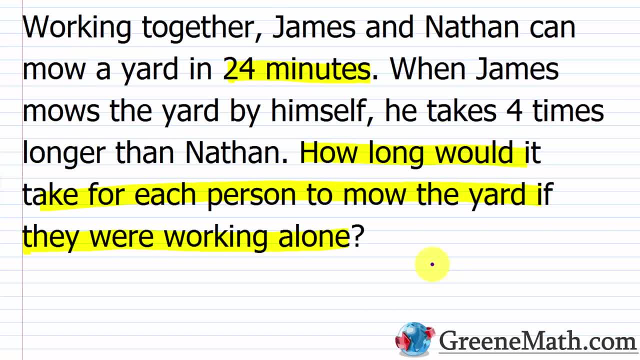 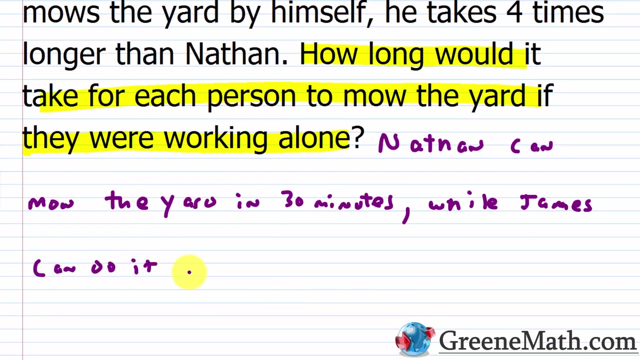 it's okay. You can put it in terms of minutes, right, It doesn't matter. So I'm just going to say that Nathan can mow the yard in 30 minutes. So Nathan can mow the yard 30 minutes. Then I'll say, while James can do it, And you can say two hours or 120 minutes, I'll 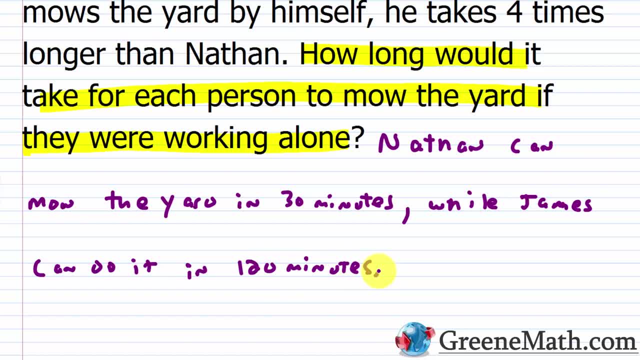 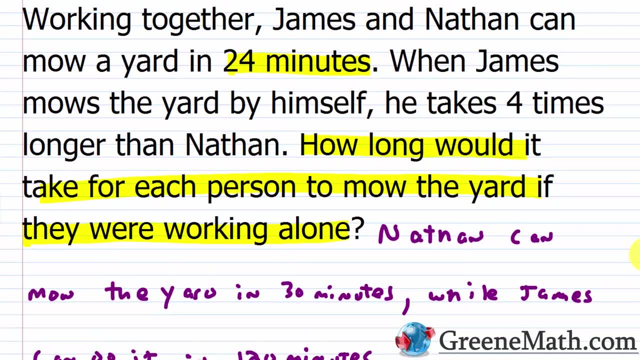 just say 120 minutes, because the problem was given in minutes. But again you can put two hours, It's the same thing. So does this make sense? Let's kind of scooch up just a little bit. So again, working together, James and Nathan can mow the yard in 30 minutes. So Nathan can mow the yard in 30 minutes. 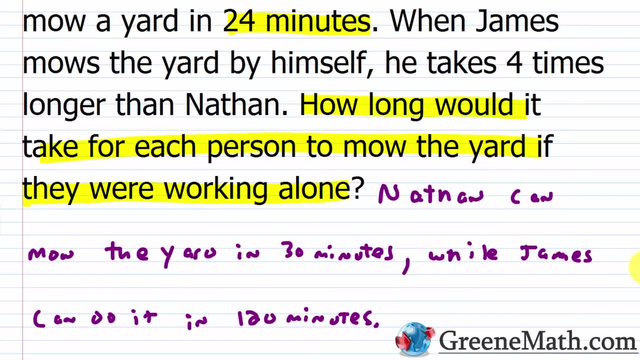 So we know that When James mows the yard by himself, he takes four times longer than Nathan. So, according to our answer, James does it in 120 minutes and Nathan does it in 30 minutes. So if this is correct, we're good to go right, Because it is four times, 30 times four will give. 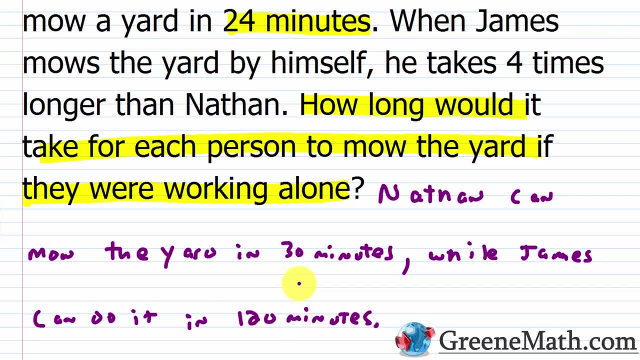 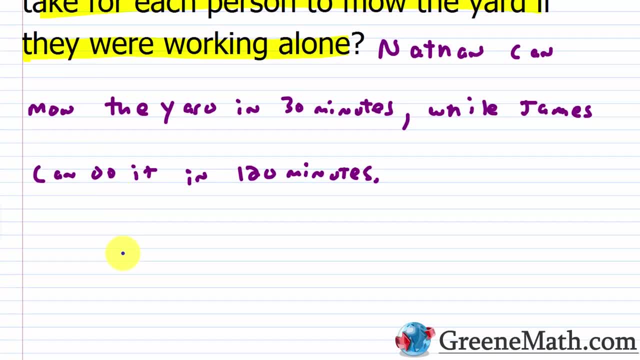 me 120.. So that part does check out. We just need to make sure that they can work together and get it in 24 minutes. So again, think about this: The amount of work that Nathan does is going to be 120 minutes. So if this is correct, we're good to go right, Because it is four times. 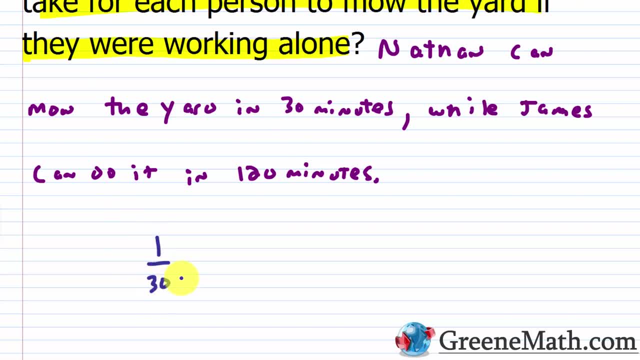 So he's going to do one over 30 of that job every minute. So he's going to do this again. if they work together for 24 minutes, Then if I add to this how much James does, So he's going to do one over 120 of that job for every minute And he's going to do that for 24 minutes If I. 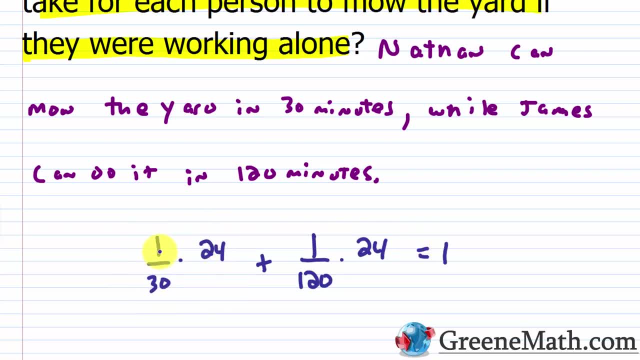 sum these amounts, I should get one. This is the amount that Nathan does all the way to the left. Then we have plus. Again we have the amount that kind of James does over here. Again, if I sum them, I should get one. So how can I reduce this here? Well, I can divide both by six. That would give me 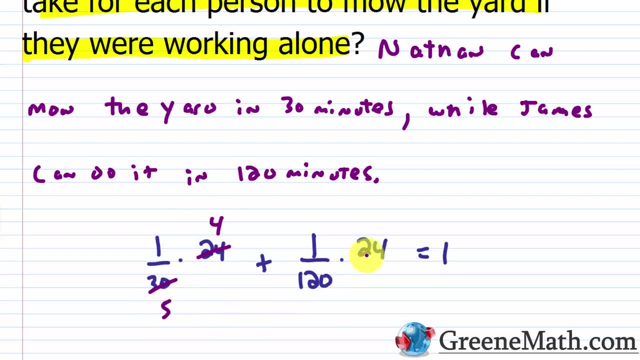 a four here and a five here. For this one, 120 divided by 24 is five, So I can cancel this with this and put a five here. So you've got four fifths of the job, which is what Nathan's going. 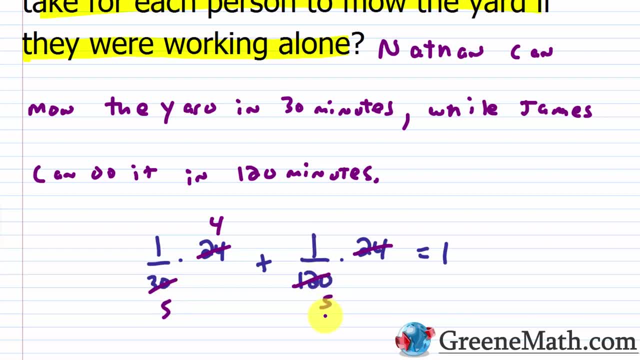 to do, plus one fifth of the job, which is what James is going to do. You sum those two amounts together, you get five fifths, or one again for one completed job. So our answer here is correct: Nathan can mow the yard in 30 minutes. 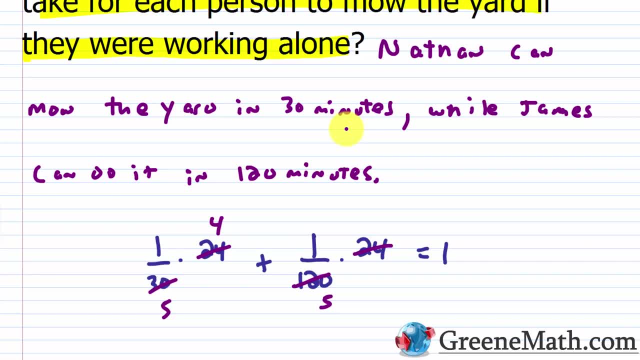 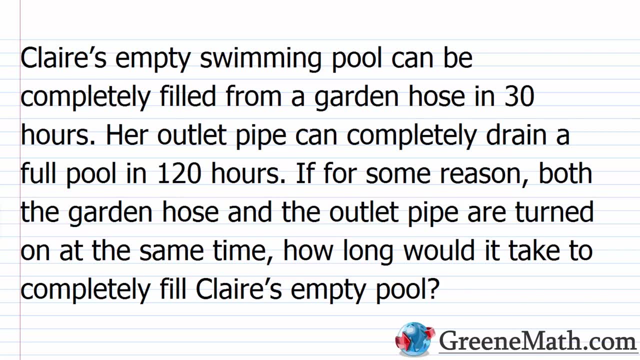 While James can do it in 120 minutes or again two hours. Okay, So pretty easy overall. Let's look at one that's a little bit more challenging, but again it's not so much because these problems are really easy. So Claire's empty swimming pool can be completely filled from a garden hose in 30. 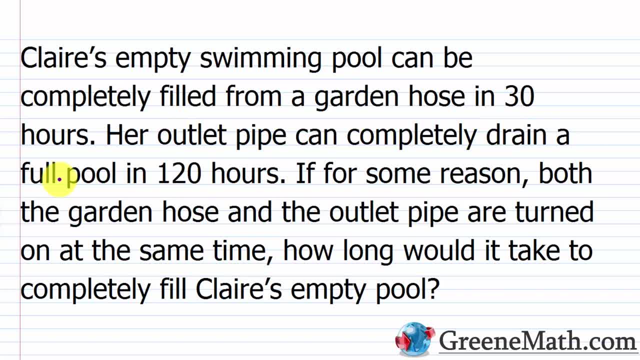 hours. Her outlet pipe can completely drain a full pool in 120 hours. If, for some reason, both the garden hose and the outlet pipe are turned on at the same time, how long would it take to completely fill Claire's empty pool? So the question we need to answer here is: how long would it take? 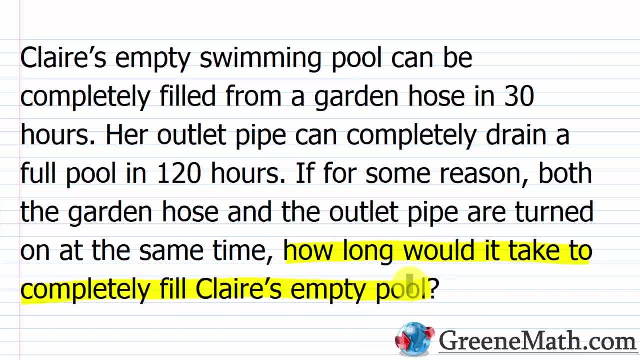 to completely fill Claire's empty pool. Given these two competing forces, you've got one kind of hose pipe that's filling the pool And then you've got an outlet pipe or you can say a drain pipe that's emptying the pool. So they're kind of working against each other. You can think about. 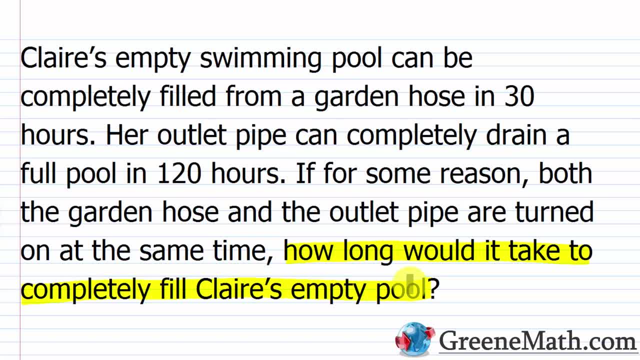 this as if you're filling your kitchen sink, Okay, And you kind of. you got the water on full blast, but you hold the stopper just up just a little bit, right? So some of the water can drain. So if the amount of water coming in is more than the amount of water going out, 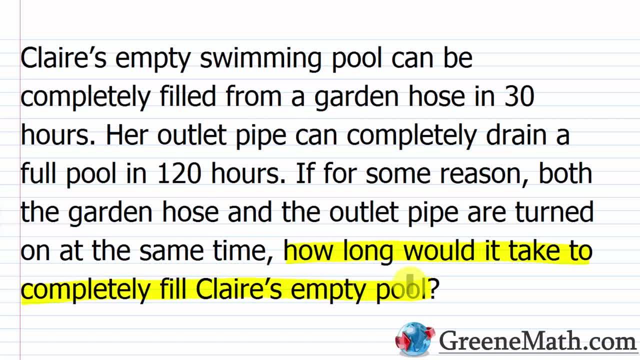 eventually you're going to fill your sink, right, But it's just going to take longer than if you had the sink kind of all the way stopped up. Okay, So that's the idea of what's going on here. So how can we model this? Let's just say we're going to let X be equal to the. 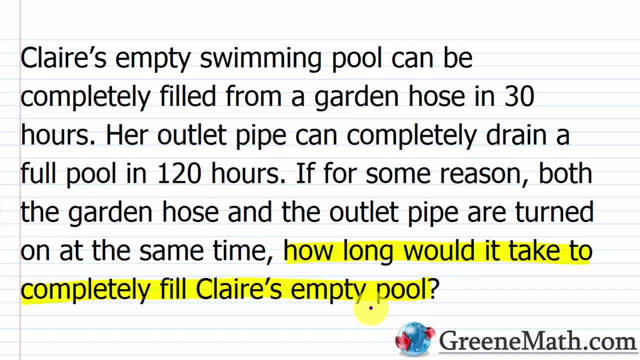 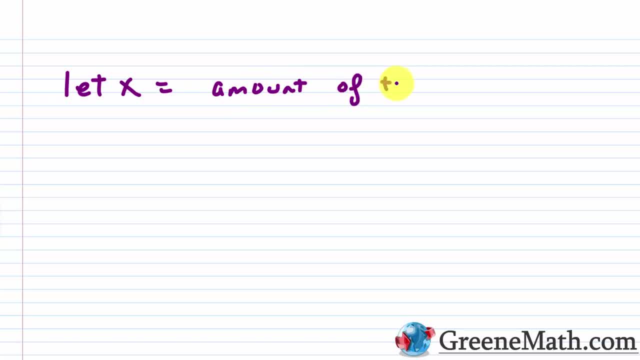 amount of time it would take to completely fill Claire's empty pool. So I'm just going to say: let X be equal to the amount of time to fill the pool. Okay, Let's go down to the kind of table. Let's organize some stuff. So we've got our hose. 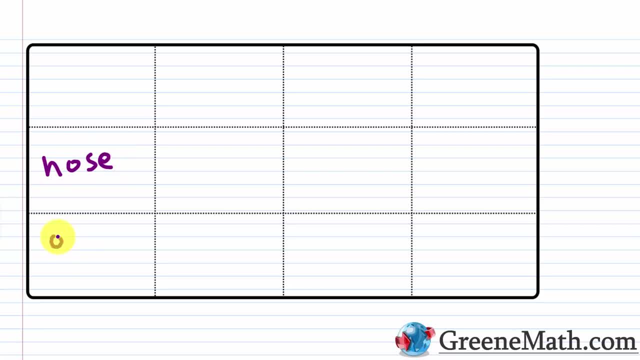 that's filling the pool, And then we've got our outlet pipe that's trying to drain it. And let me be more specific here and just put garden hose. So garden hose, because that's what it says in the problem. Now again, we're going to have 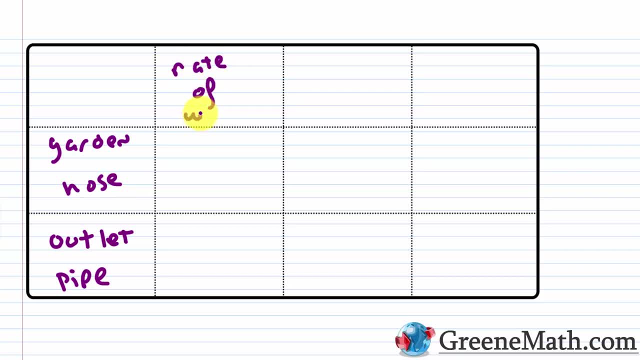 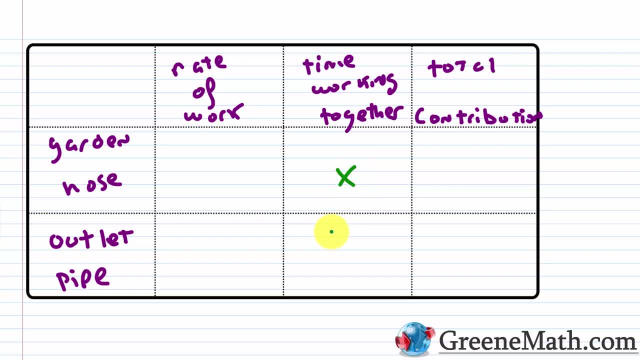 So we know one thing so far: it's the time working together And then we're going to have our total contribution. There's X because we just let a variable represent that. So this is X and this is X The rate of work. let's go back up. 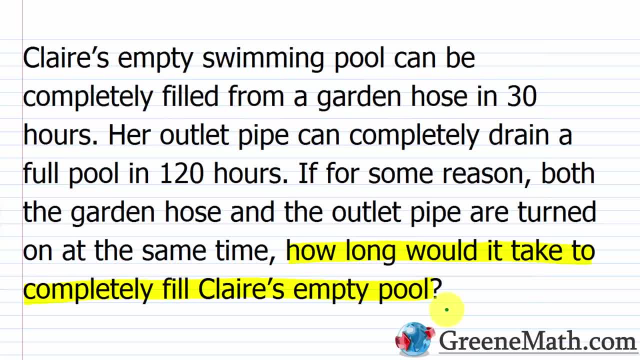 We've got to find the garden hose and the outlet pipe So the garden hose can fill the pool in 30 hours. So every hour it's done one over 30 of that job. So the rate of work is one over 30.. 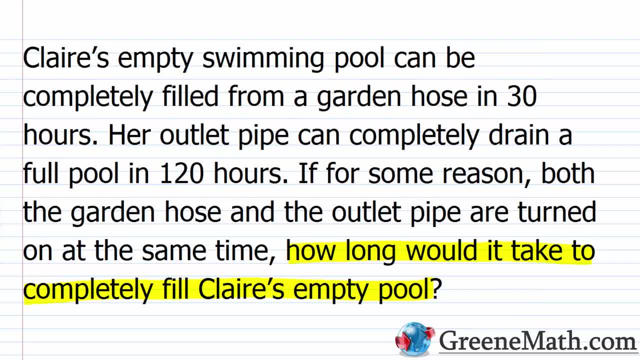 So I'll put one over 30.. Now the outlet pipe which is trying to drain the pool. that's its goal. okay, So every hour, since it takes 120 hours to do this, it's done one over 120 of that. 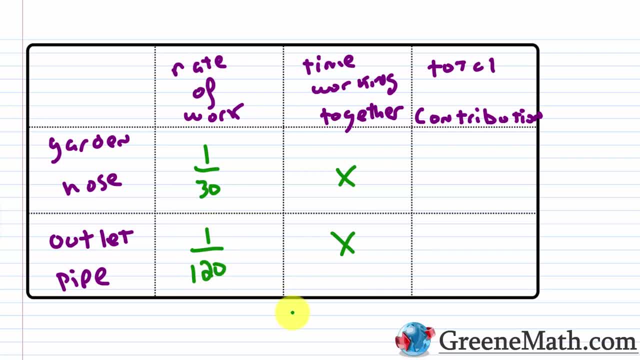 So I'll put one over 120.. So that's the rate of work. Now the contribution works a little bit differently here because they're competing forces, right? You can kind of think about the garden hose as filling it. So I'm going to put a positive one over 30 times X. 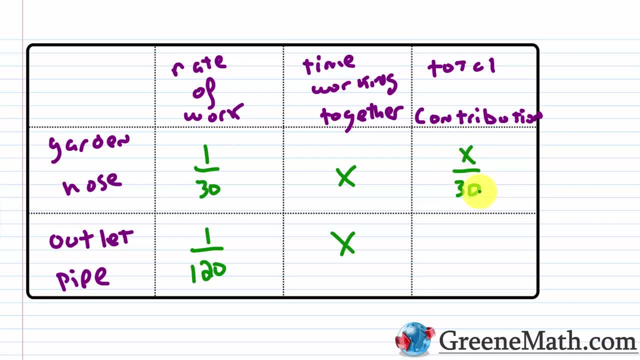 or you can just put X over 30.. Really, you can think about the outlet pipe as fighting against this right. You can think about what it's doing as subtracting away, So you can put this as a minus X times one over 120,. 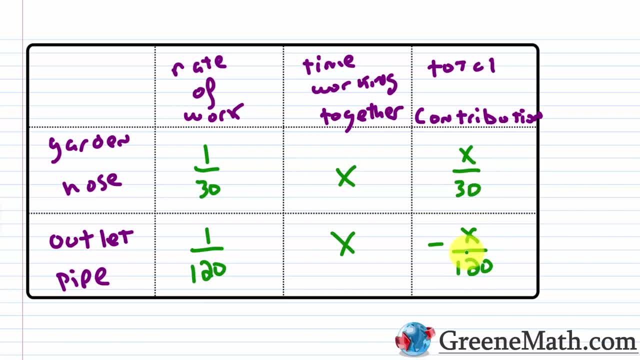 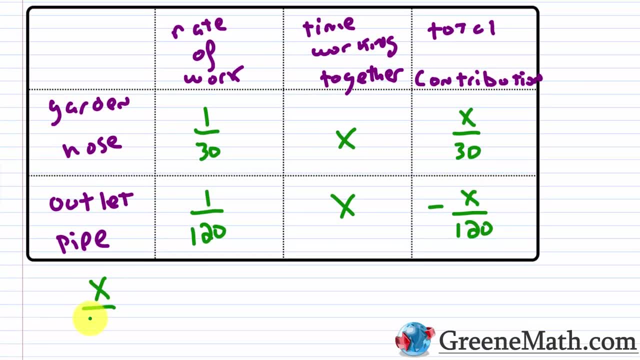 which would be X over 120.. So if you sum these two amounts together, you should set it equal to one and solve that equation. So I would have X over 30.. I'll just put minus or you can put plus negative. 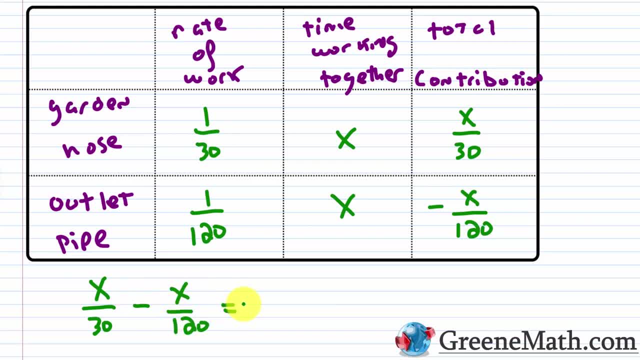 doesn't matter, I'll put minus X over 120.. I'll set that equal to one. So in other words, the total contribution or the total amount of water that goes in from the garden hose, minus the total contribution or the total amount of water. 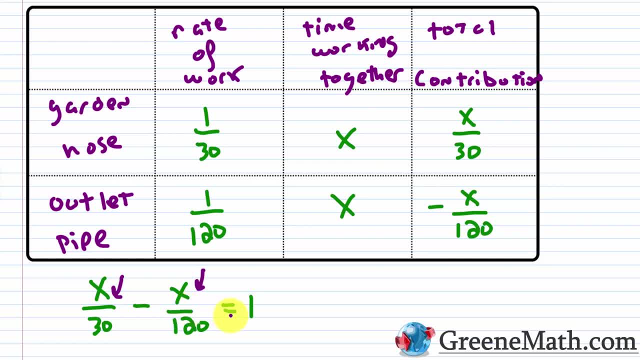 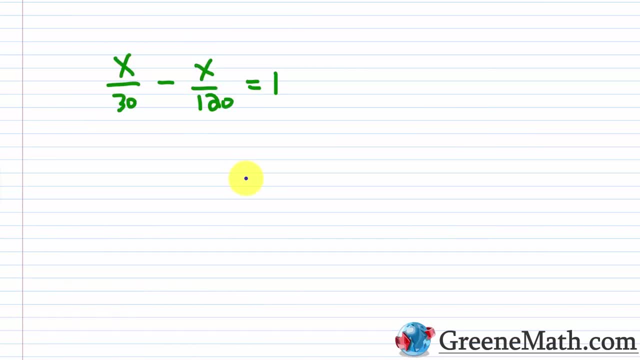 that gets pulled out from the outlet pipe. when that's set equal to one, the value for X is going to tell me the amount of time it takes for them to complete that job again working together. So let me copy this. So what I want to do is just multiply both sides by the LCD. 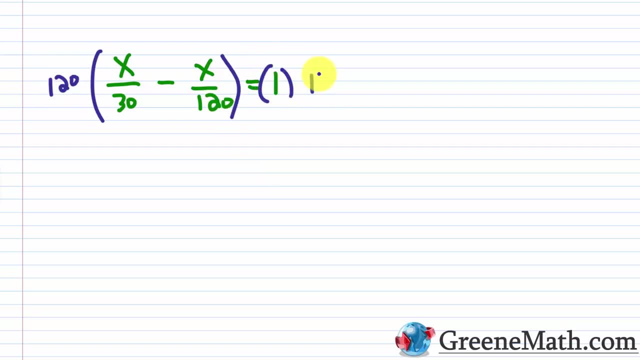 which is going to be 120.. Pretty easy to do, So I know that I'm going to distribute this to each term inside the parentheses: 120 divided by 30 is four, right? So I'd have: 4X minus 120 divided by 120 is one. 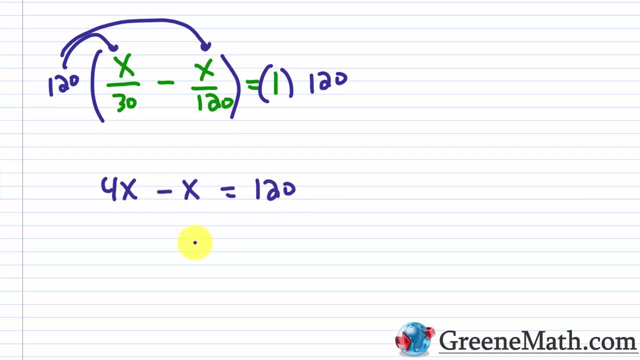 So I just have X there. This equals 120.. 4X minus X is 3X. This equals 120.. Divide both sides of the equation by three And you're going to find that X is equal to 40. So that tells us what. 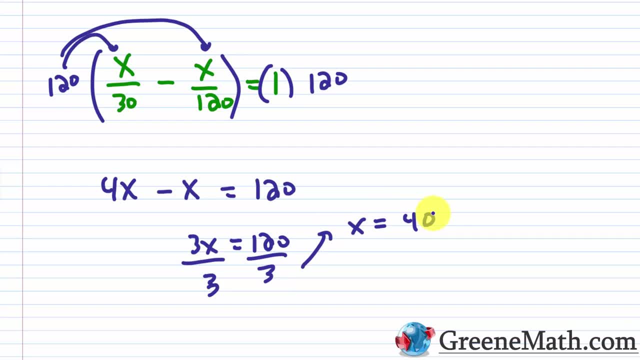 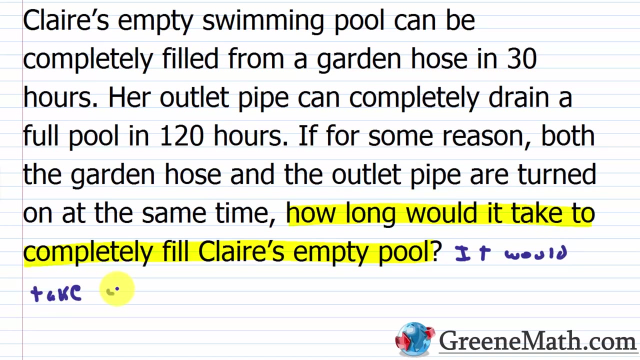 It tells us that the garden hose and the outlet pipe can both be left on And the pool is going to go from completely empty to completely full in 40 hours. Let's go back up. So it would take 40 hours to fill the pool. 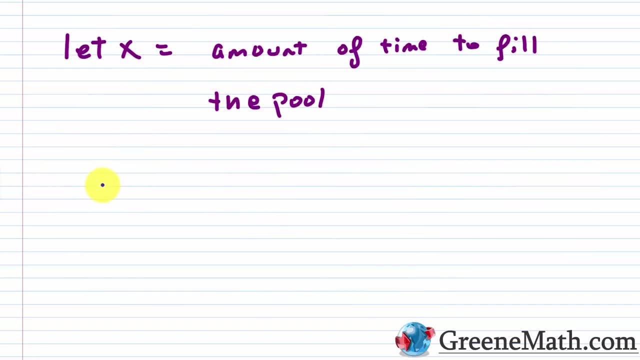 Okay, So let's check this. So again, I go back to my formula of A equals R times T. So think about this. for each scenario You have another one over here. So what I'm going to do is I'm going to say the garden hose. 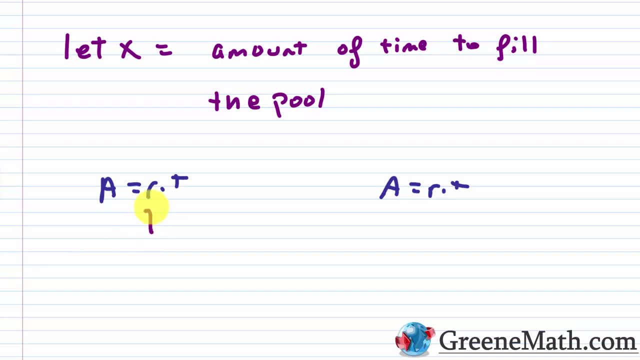 how much water does it put in? So we think about the rate Again. it does a full job in 30 hours, So the rate is one over 30. When they work together again, they're going to work for 40 hours.